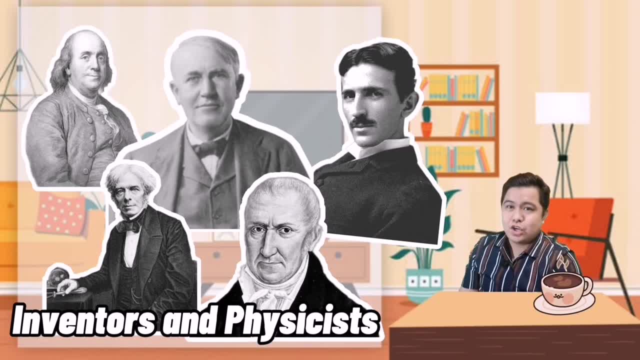 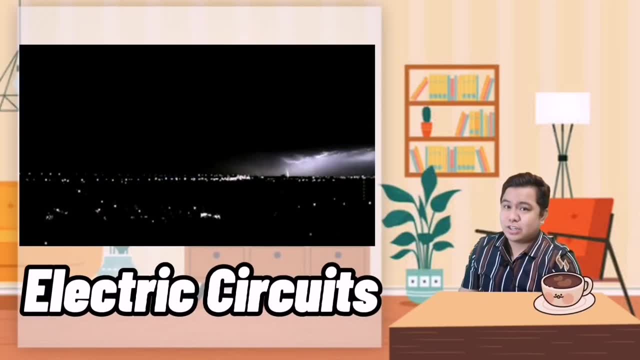 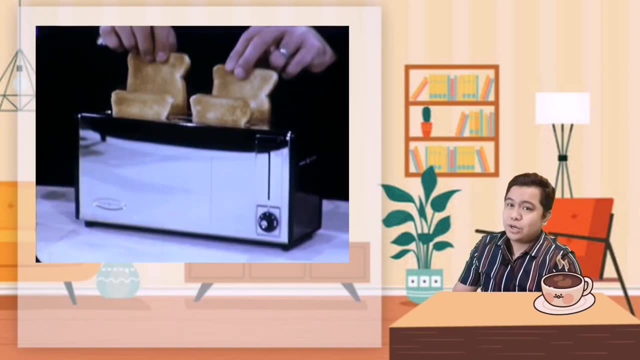 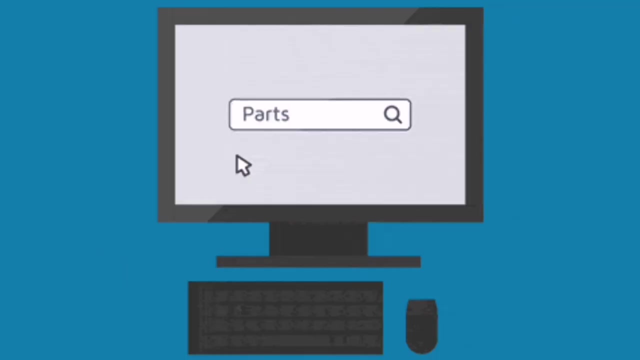 Faraday and other inventors and physicists who devoted their life in studying and use their knowledge of current conductivity and electric circuits to create the light bulb and other technologies related to electricity. we were able to find the you And you are able to watch me through this video, because computers or mobile phones are. 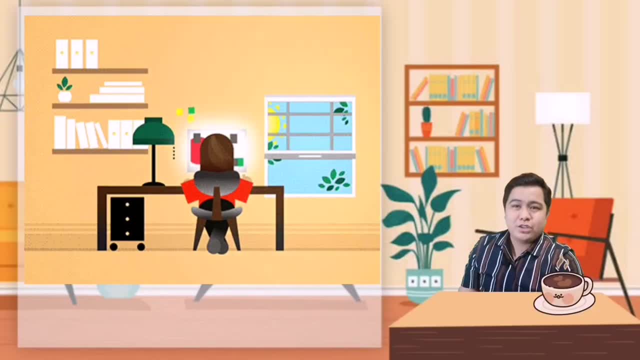 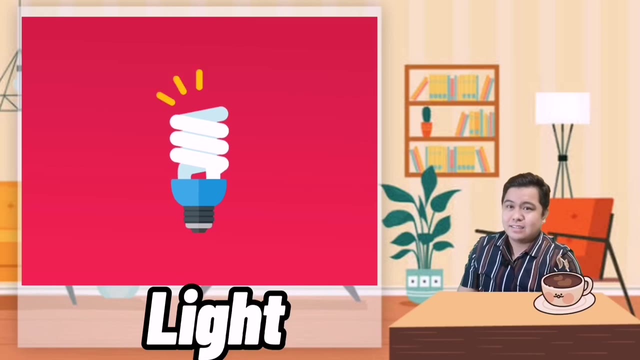 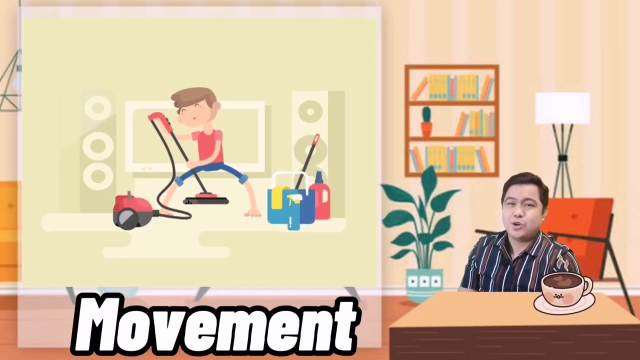 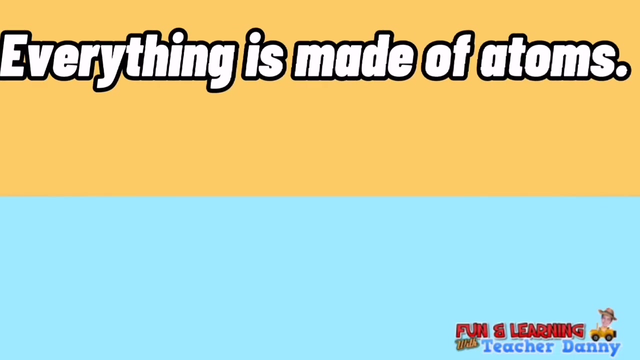 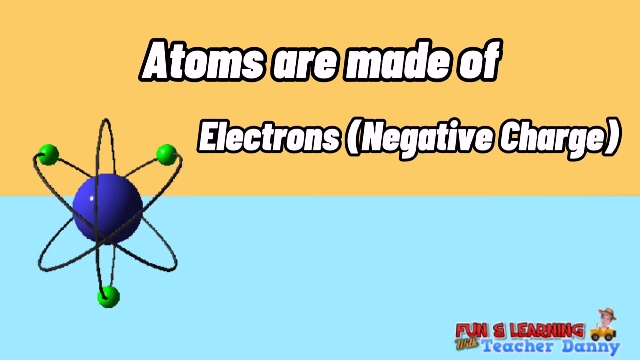 charged with electricity. We use electricity every day in almost all gadgets and other objects all around us. Electricity can produce heat, light, sound and energy. But how is it made? Remember that everything is made of atoms. Well, atoms are made of electrons, which are negatively charged, protons, which are positively. 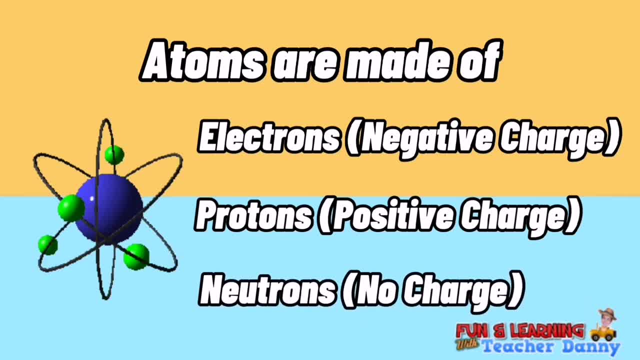 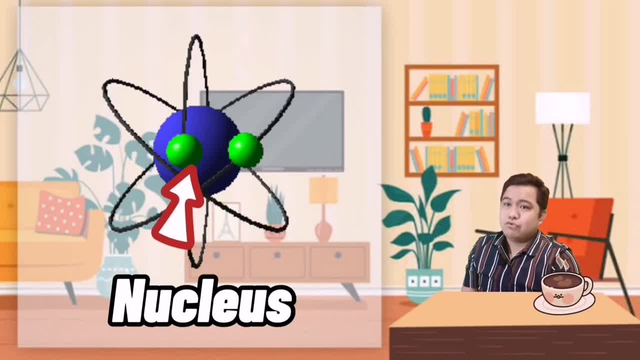 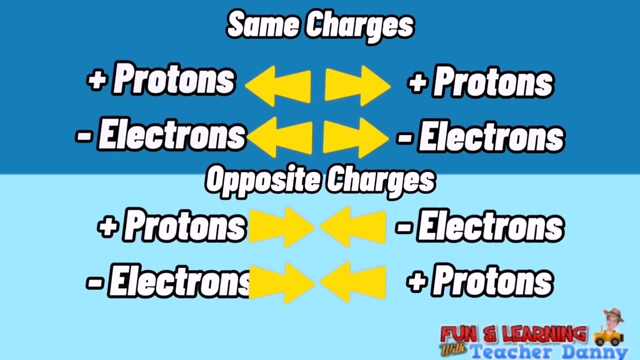 charged, and neutrons, which has no charge. Now, the center of the atom contains a nucleus, which is the nucleus. The nucleus is made of neutrons and protons. Now take note that the same charges repel each other or move away from each other, while 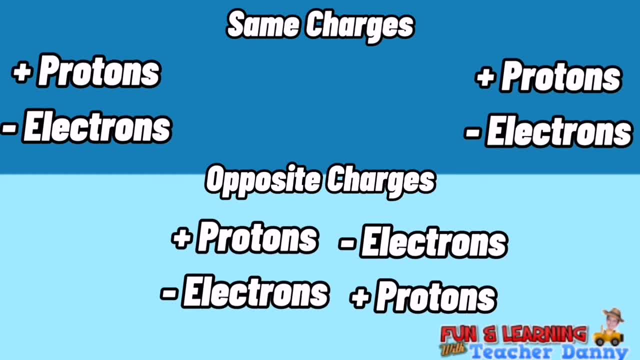 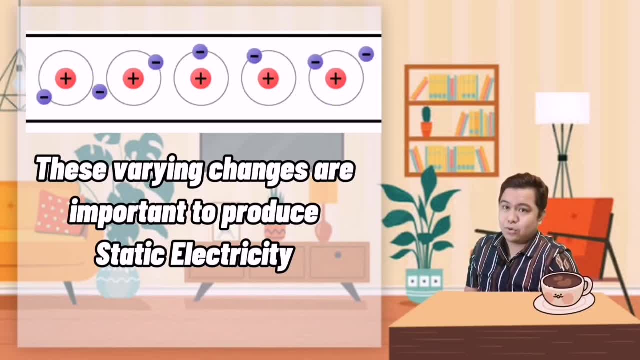 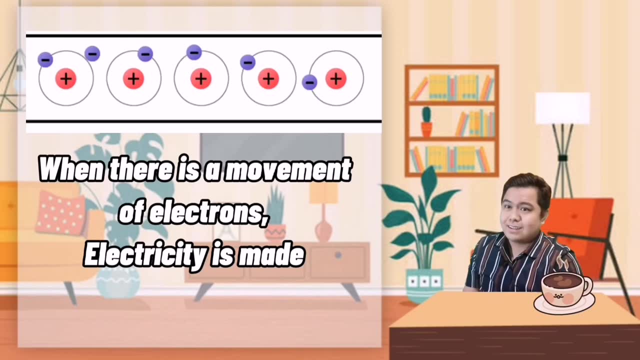 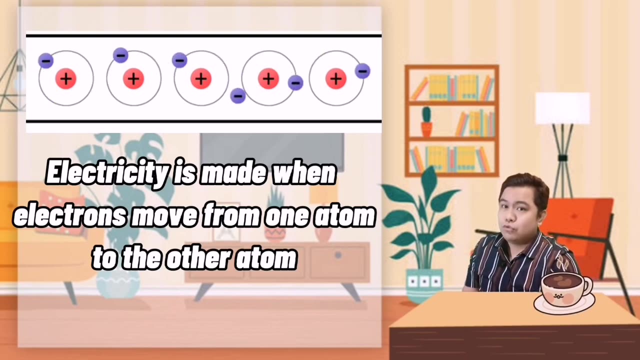 opposite charges attract each other. Now these varying changes are important so that static electricity can be produced. Now, when there is a movement of electrons, electricity then is made Again. electricity is made of electrons. Electricity is made when electrons of the atom move from one atom to another. 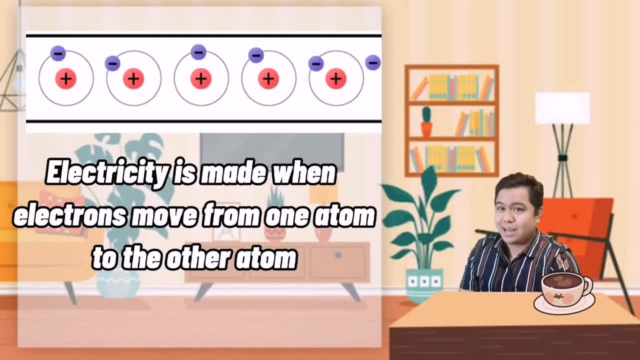 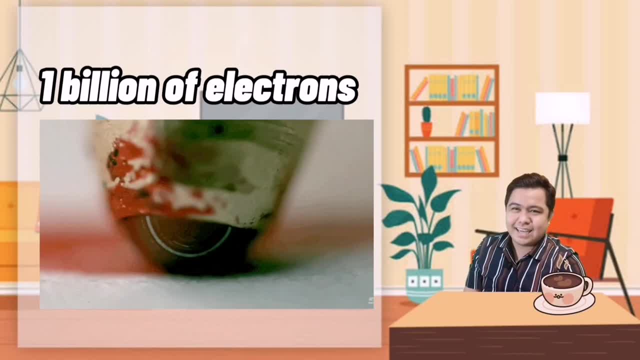 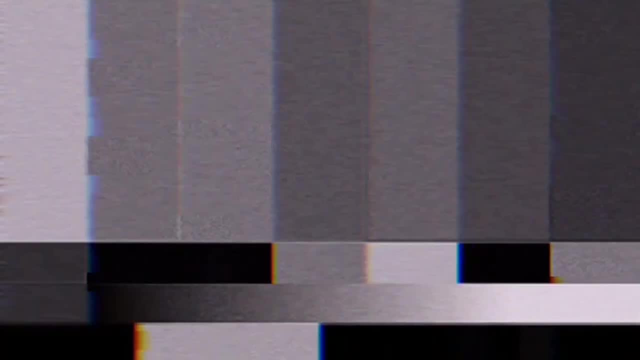 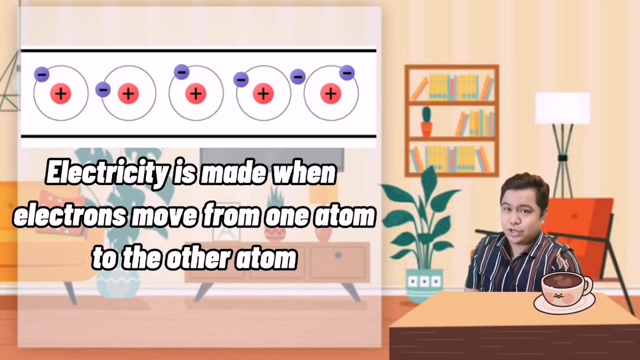 Imagining this would give us an headache. But to visualize, 1 billion of electrons can fit into a ball that is at the tip of a ball pen. Can you imagine that? What Now? as mentioned a while ago, Electricity is produced when electrons are transferred. 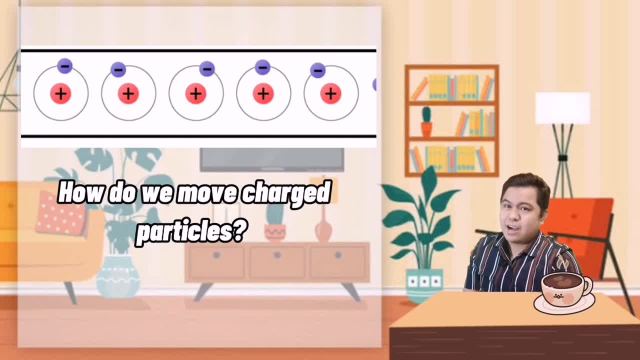 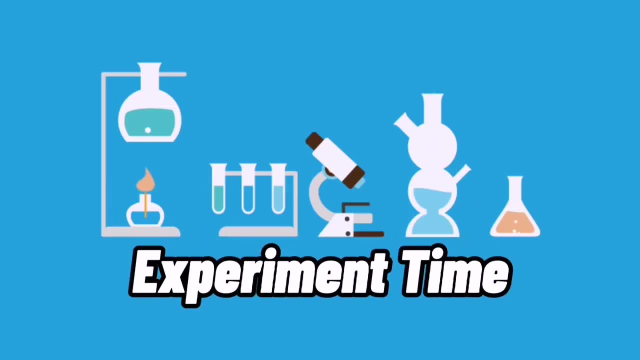 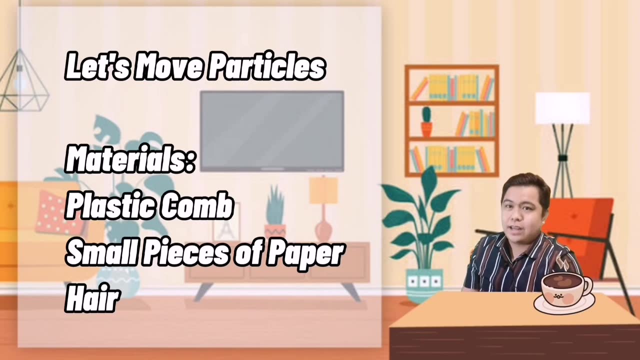 Now, how are electrons being transferred? How do we move charged particles? Now, let's have a short experiment Now. using plastic comb, small pieces of paper and your hair, we will try to move particles without touching them. Now, here's what we are going to do. 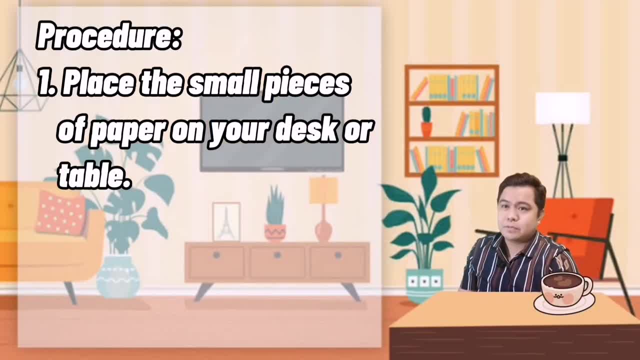 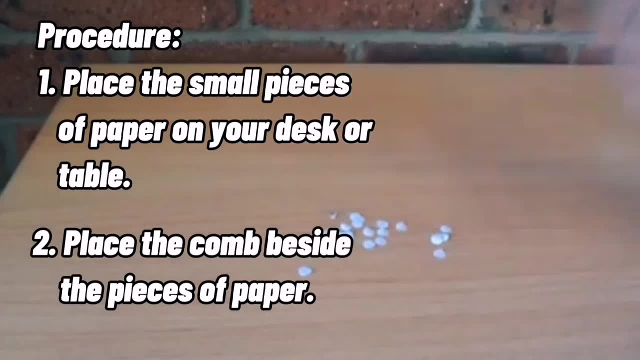 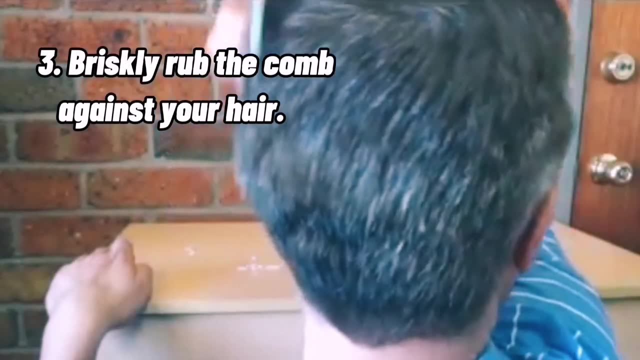 First, we place small pieces of paper on your desk or table. Second, you place your comb beside the pieces of paper. then you observe: Is there any movement? Now briskly rub the comb against your hair. Then try to put the comb near the pieces of paper. 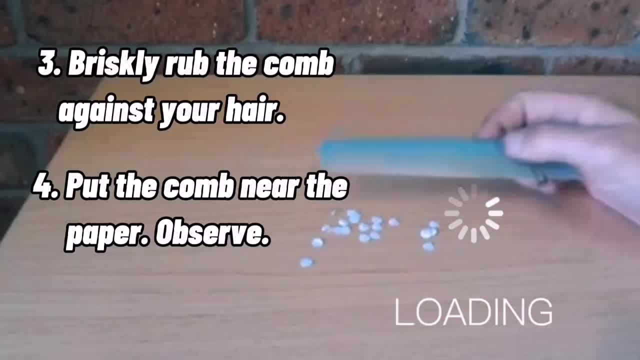 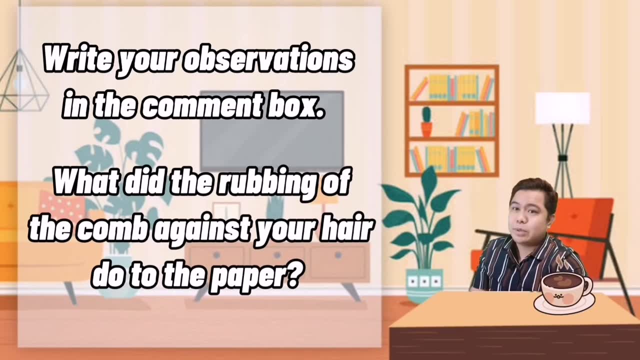 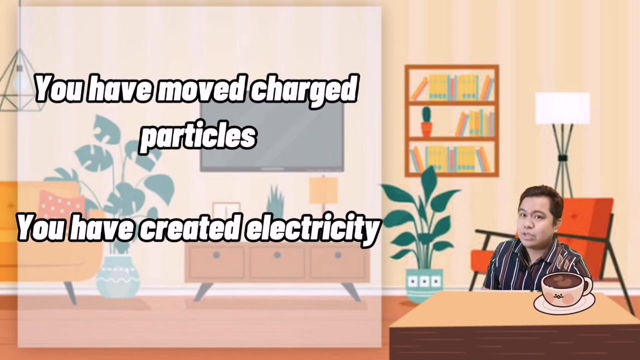 1. Now I would like you to write your observations in the comment box below. Now, what did the rubbing of the comb against your hair do to the paper? If you triumphantly did the experiment a while ago, it means that you have moved charged particles and you have created electricity, as we have mentioned. 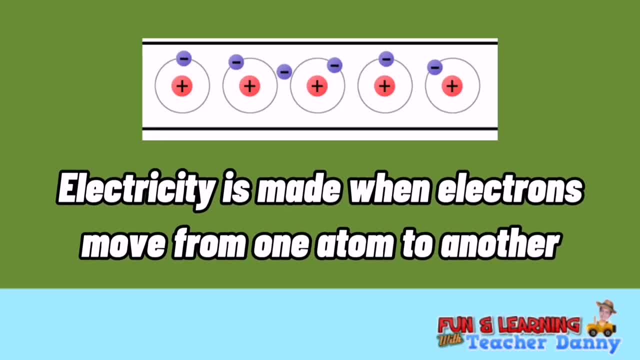 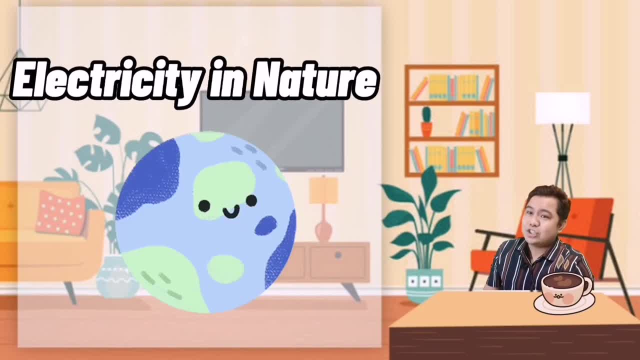 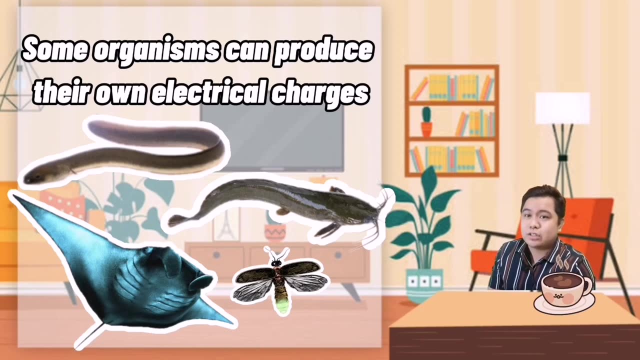 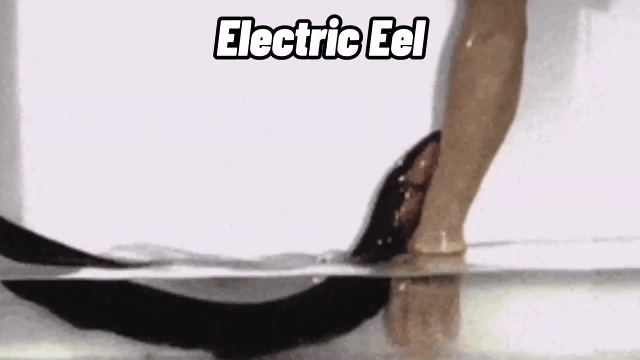 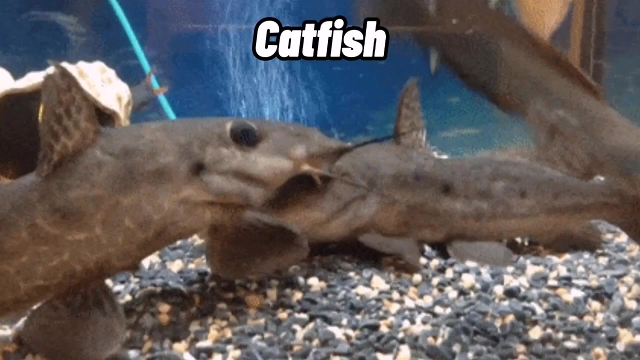 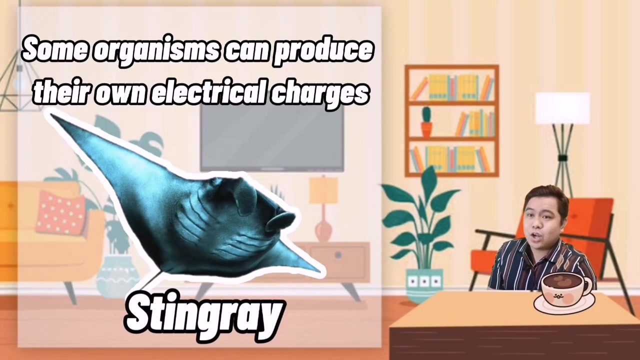 Now, electricity is made when electrons move from one atom to another. Now in nature there are different types of electricity. Some organisms can produce their own electrical charge. Electric eels, Catfish, Fireflies, Stingrays are some animals which can produce electrical charges. 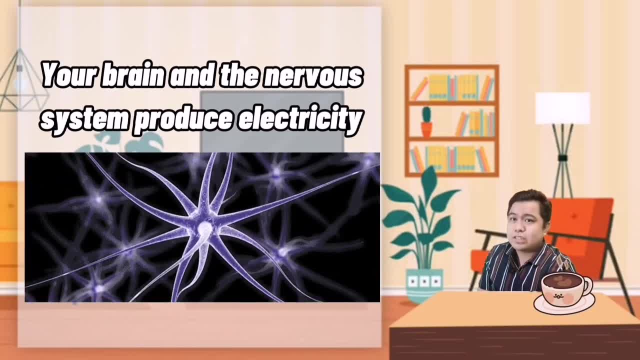 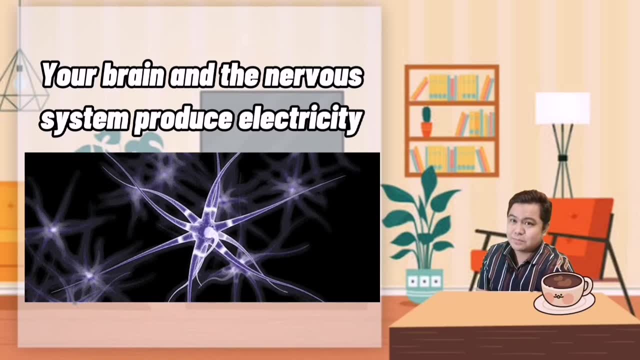 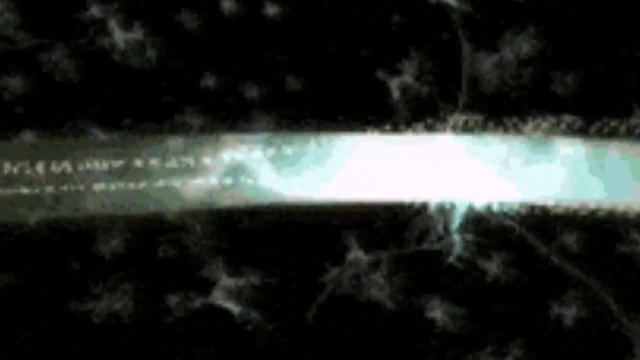 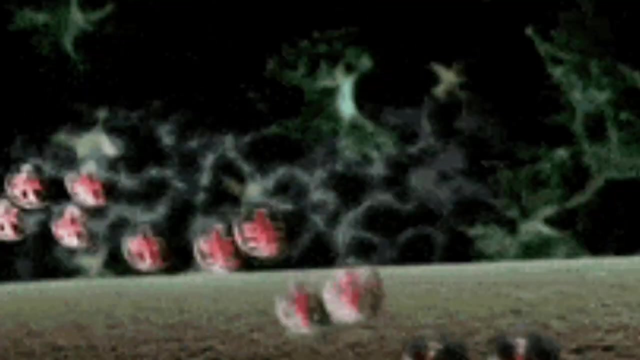 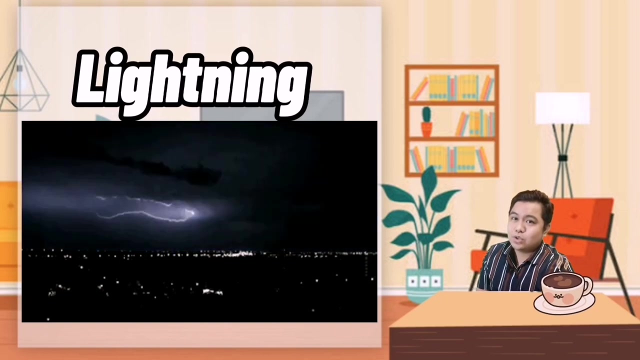 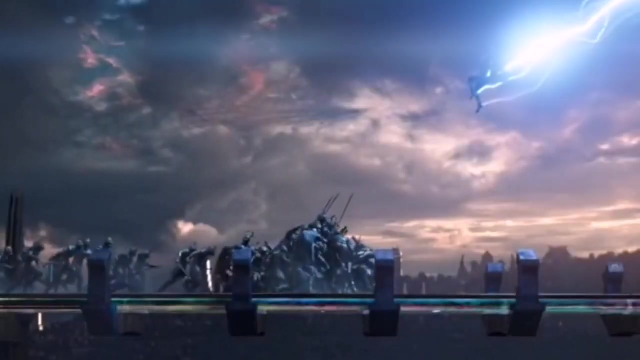 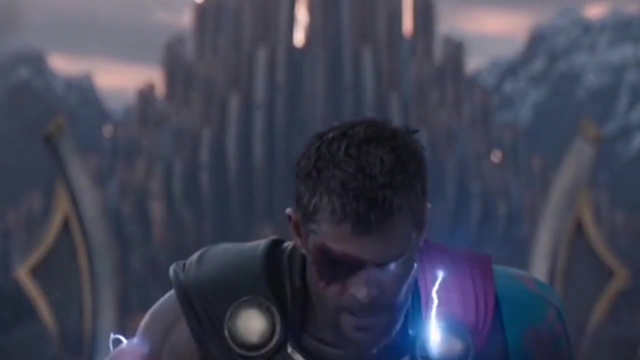 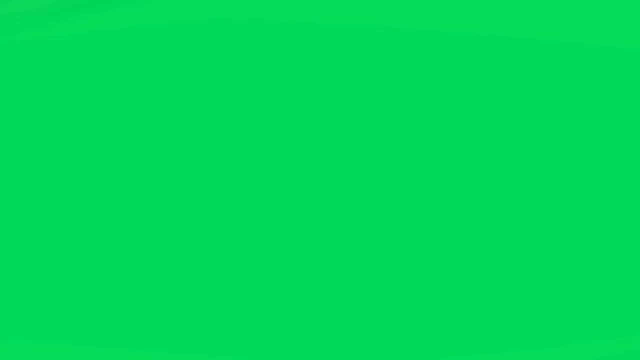 Your brain and the nervous system produce electricity also. That's why information from your sense organs are transferred in impulses. Life is also a form of natural electricity. Thank you for watching Now when there is a building of stationary electrons on a surface of an object. 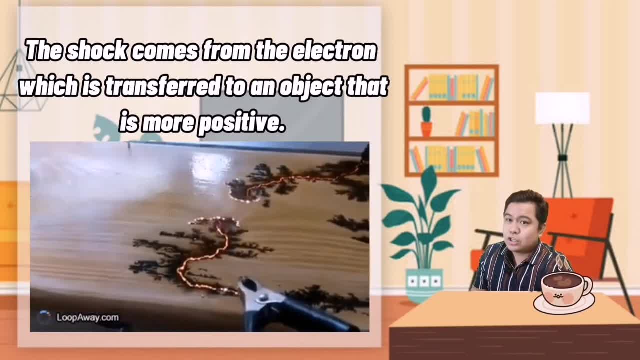 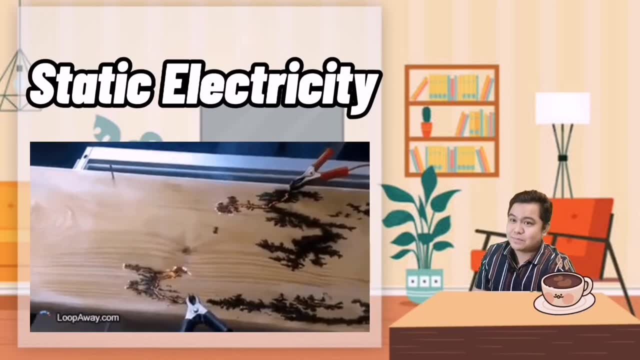 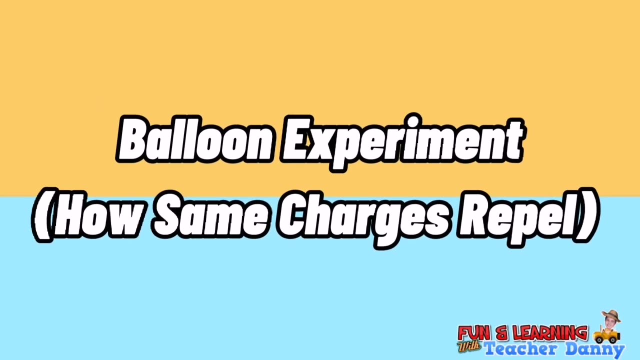 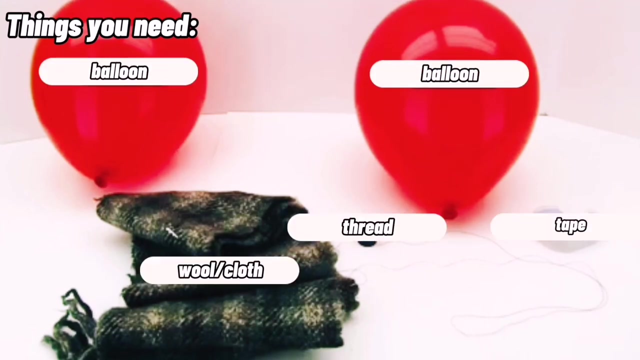 the shock comes from the transfer of electron to an object that is more positive. Now, this is what we call as static electricity. Now, it's much better than static electric current. By all means, try this method Now: your brain when it is disturbed, and crisis when you get disturbed. 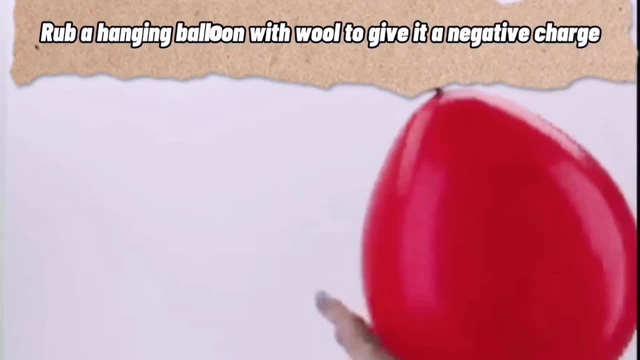 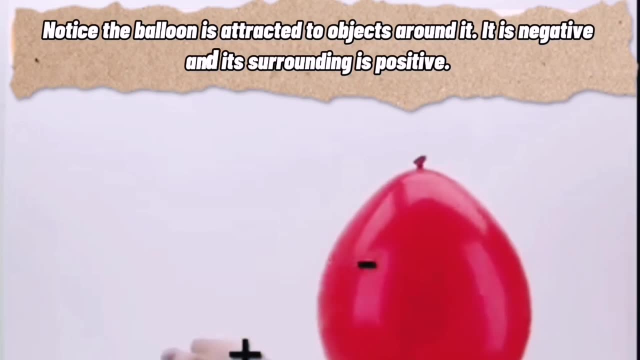 And then you can release the intent. You are making a device which makes an Receiver Receiver, so you can have your own system of behaviors to make power of your computer. All right, See you in a hectare. See you again. See you again. 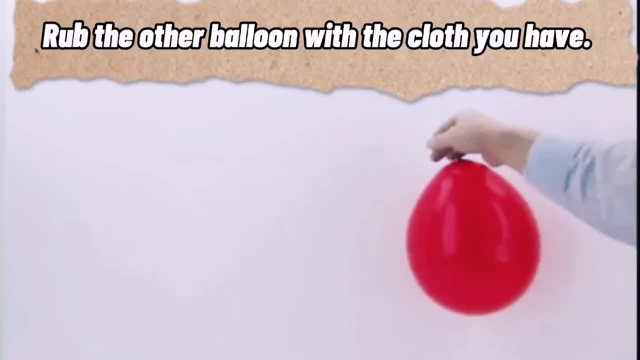 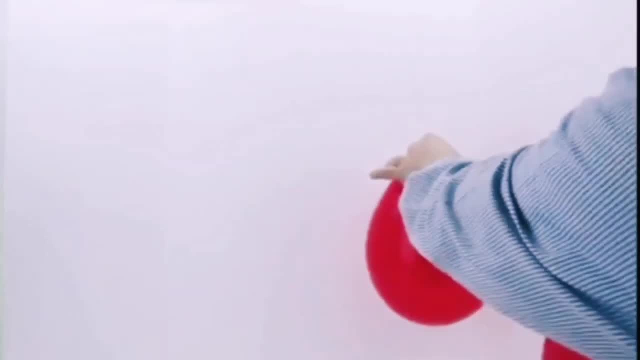 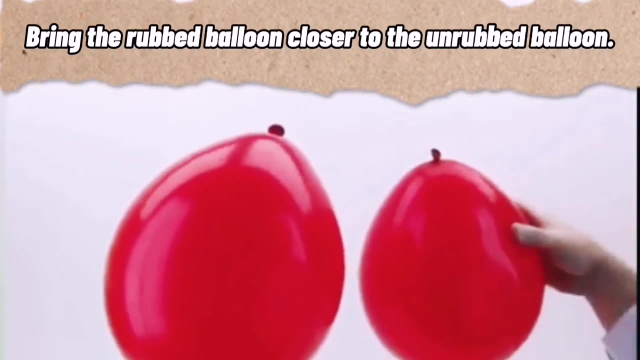 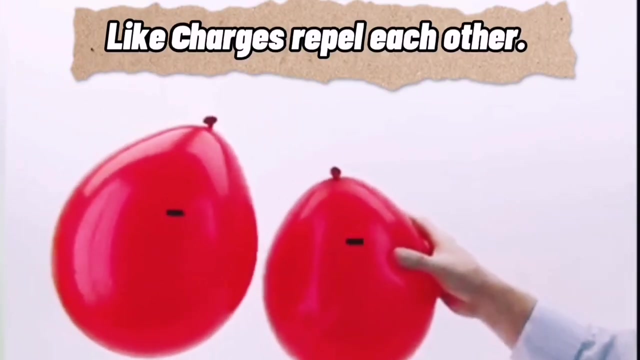 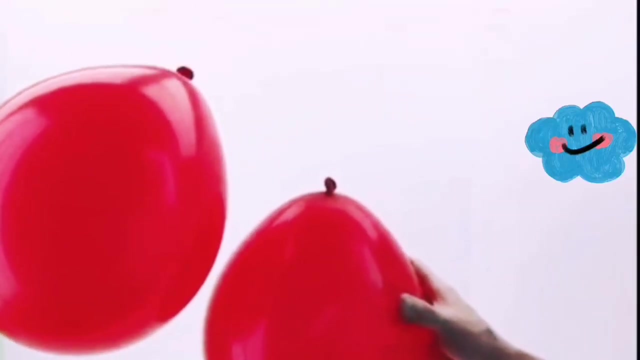 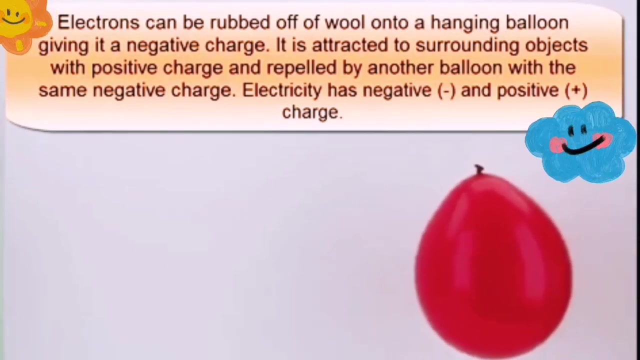 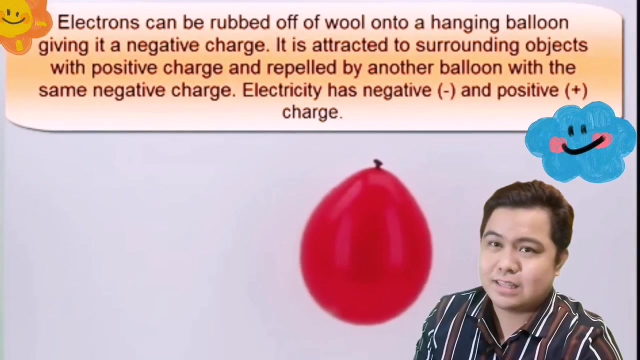 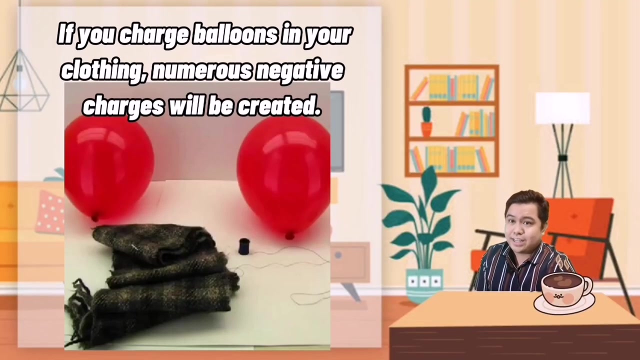 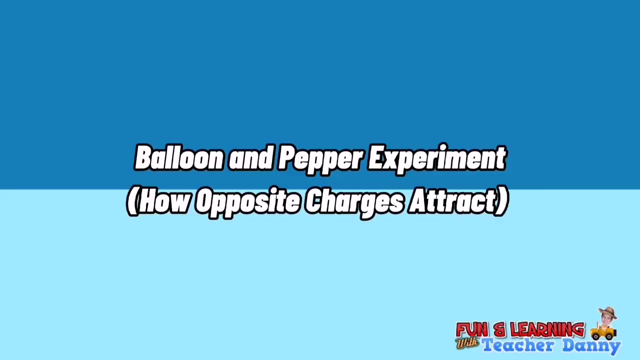 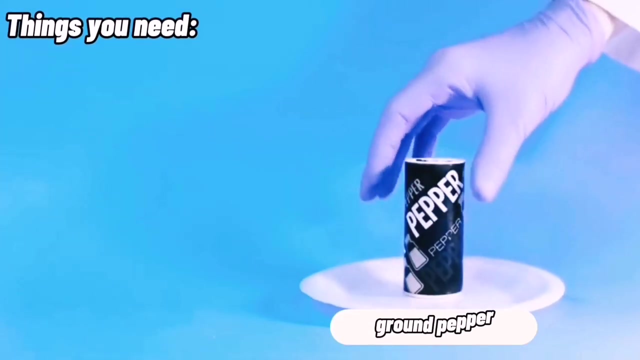 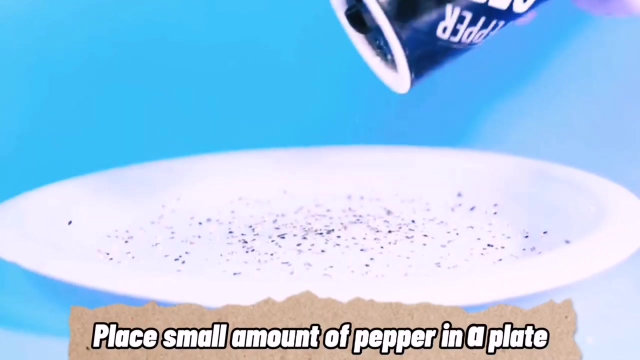 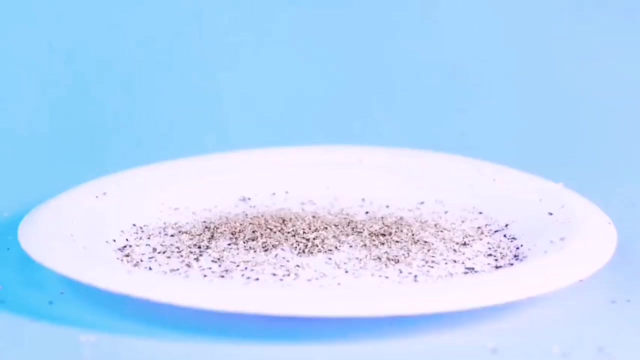 See you again, Thank you. Now, if you charge two balloons, by rubbing them on your clothing, numerous negative charges will be created. Now, the balloons will repel each other because of the number of negative charges. Now, the balloons will repel each other because of the number of negative charges. 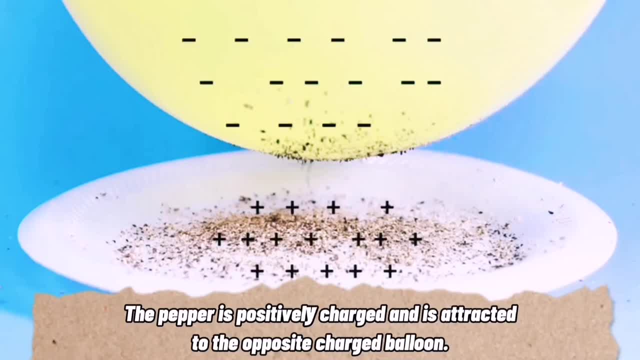 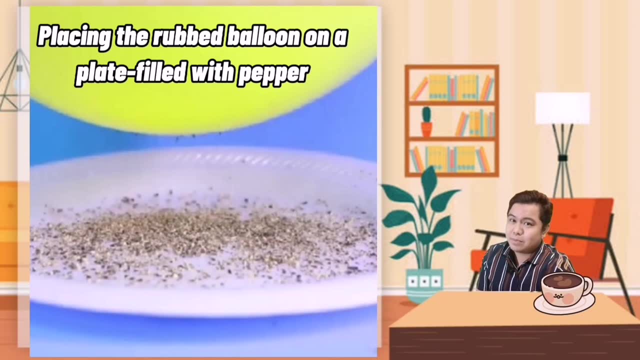 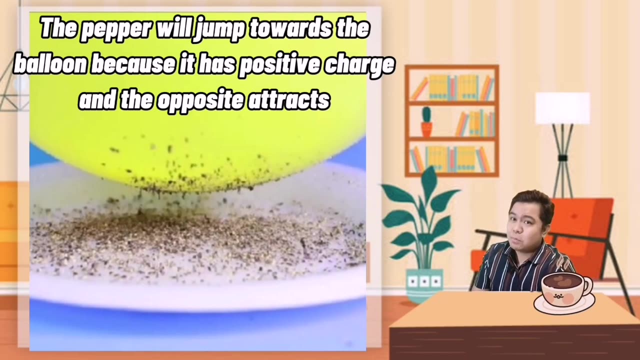 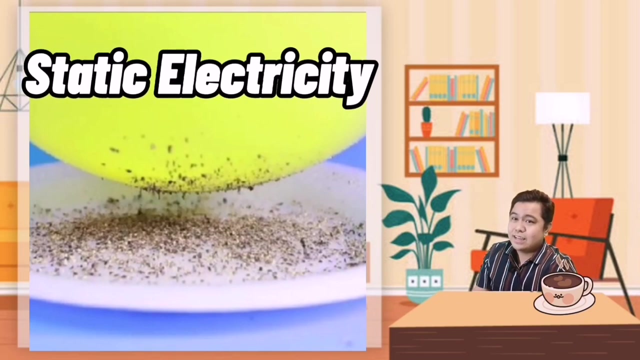 Now, if the balloon is negatively charged and you have pepper on a plate, the pepper will jump towards the balloon because it has positive charge and the opposites attract. Now this is a kind of static electricity. Now take note that there are two ways to produce static electricity. 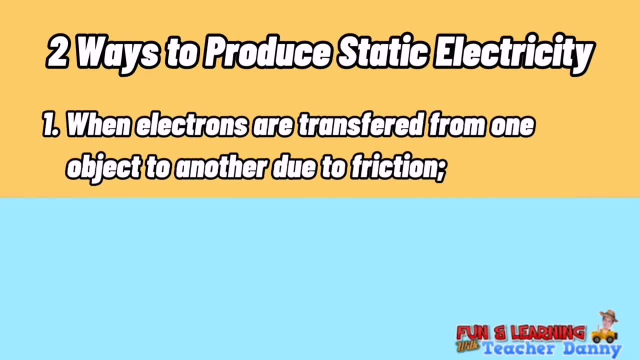 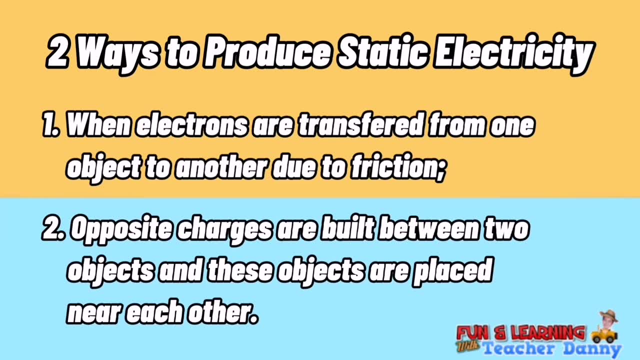 One is when you have a balloon. One is when you have a balloon. One is when you have a balloon. One is when electrons are transferred from one object to another due to friction or by rubbing, And two opposite charges are built between two objects and these objects are placed near each other. 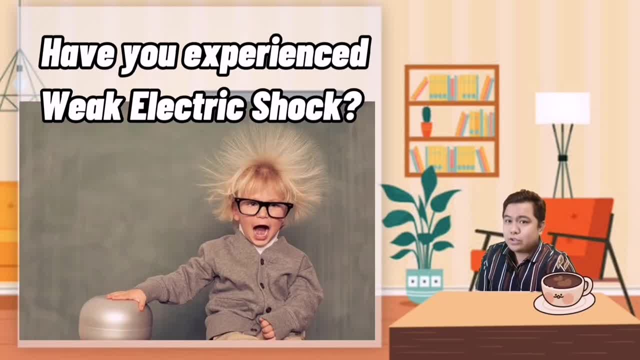 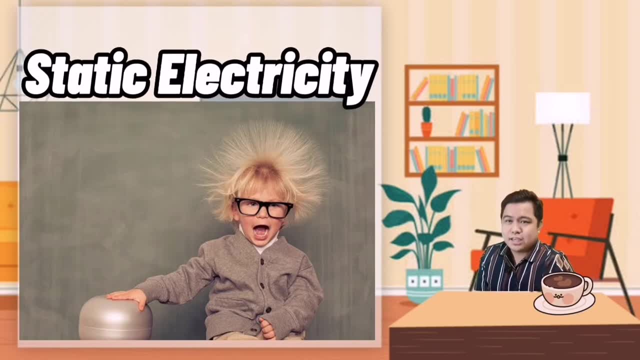 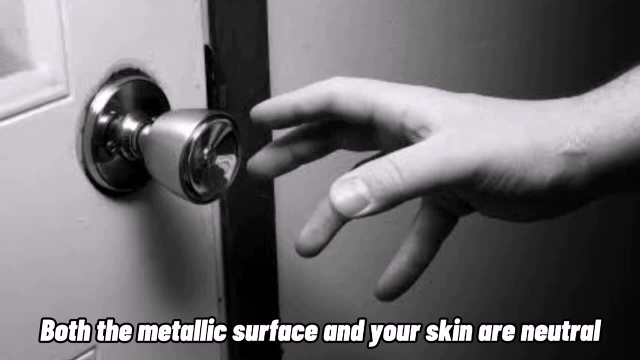 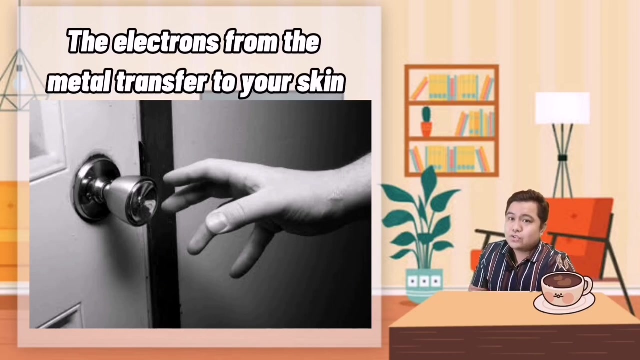 Now have you experienced a weak electric shock when you unexpectedly brush your skin to a metallic surface? Now, this phenomenon is also static electricity. Both the metallic surface and your skin are neutral, But when you unexpectedly brush your skin against the surface of the metal, the electrons from the metallic surface transfer to your skin. 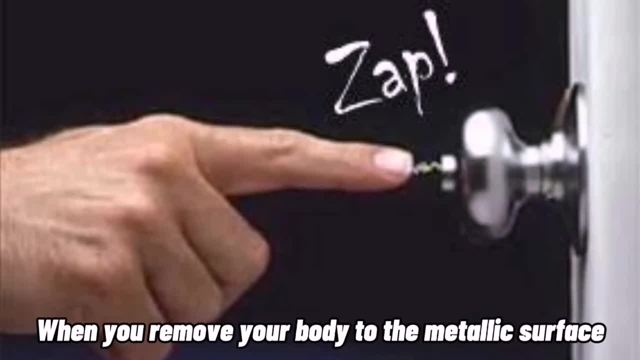 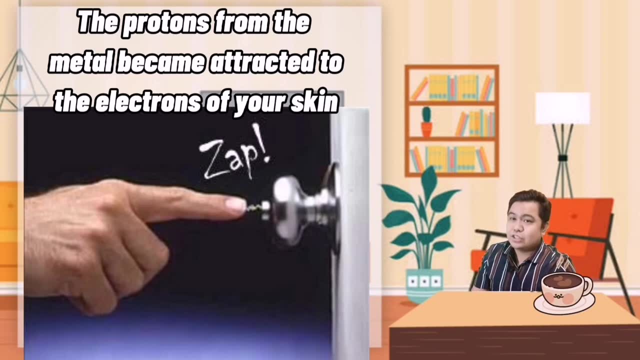 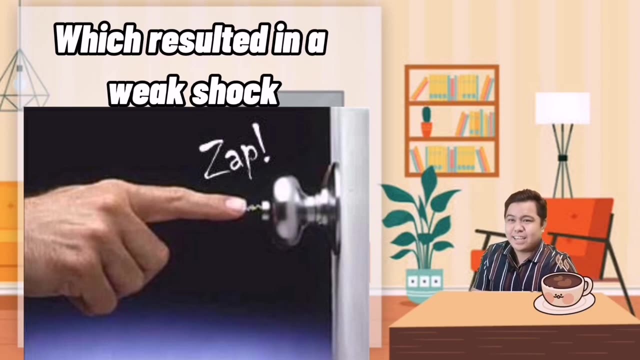 Now, when you remove your body to the metallic surface, the positive charges or the protons of the metallic surface became attracted to the electrons of your skin. Now this phenomenon is also static electricity, Which resulted in a weak shock. Hence it does show that there is static electricity in nature, right? 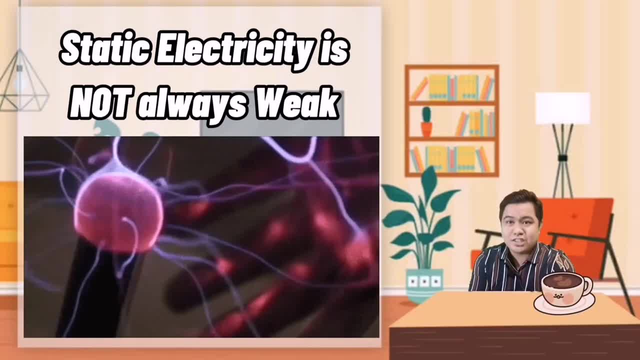 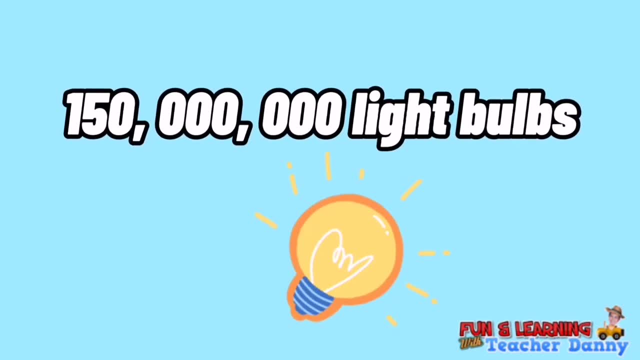 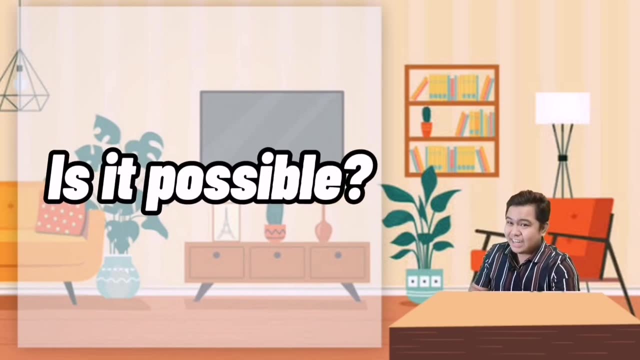 Now, did you know that static electricity is not always weak? Sometimes it can power up to 150 million light bulbs in just one strike. Do you think it is possible? Yes, that is true, Because lightning, Lightning, Lightning is a very powerful static electricity. 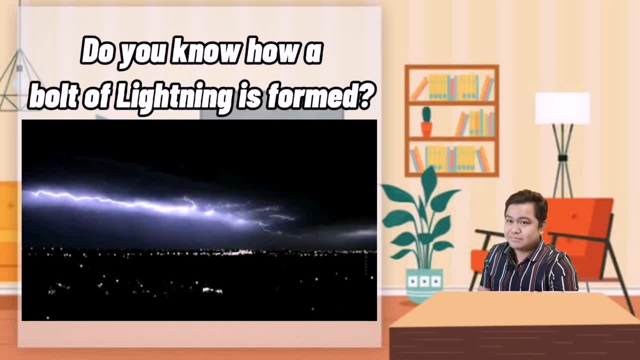 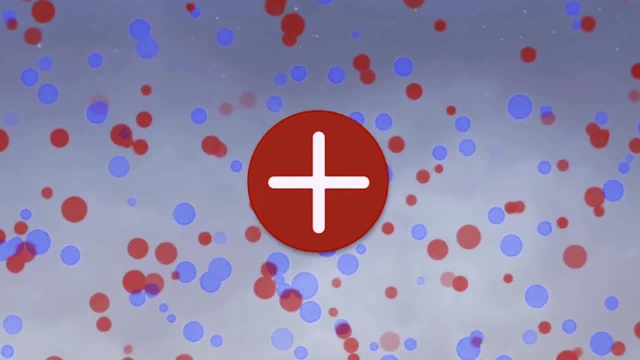 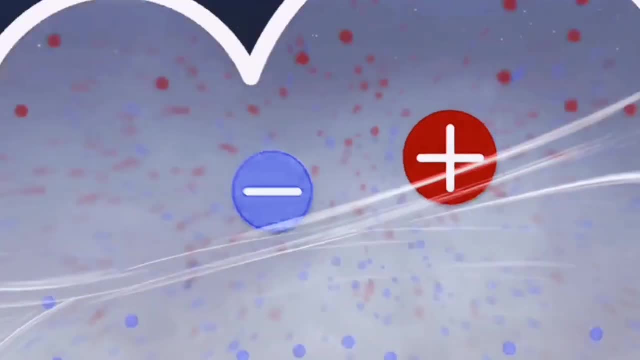 But do you know how a bulk of lightning is formed? Good, Now listen. When wind particles of the clouds rub against each other, they become oppositely charged. Now, electrons from negatively charged clouds will then quickly drop towards the positively charged clouds. 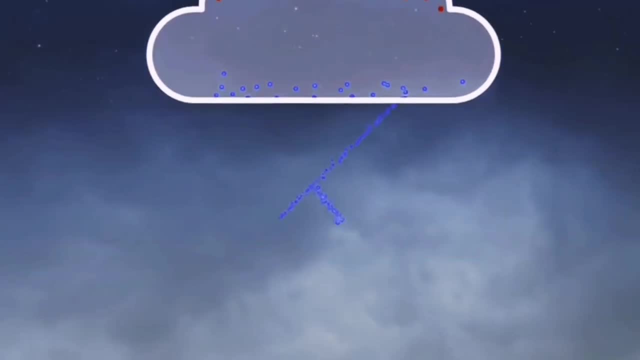 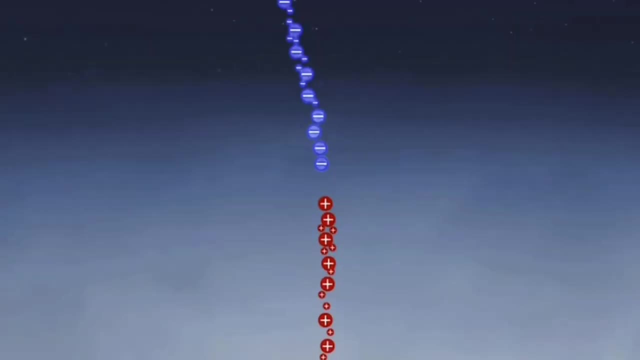 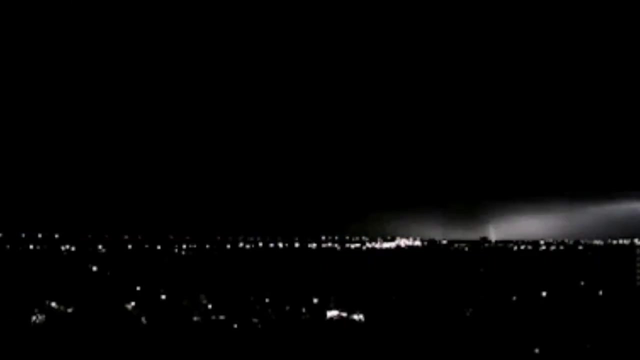 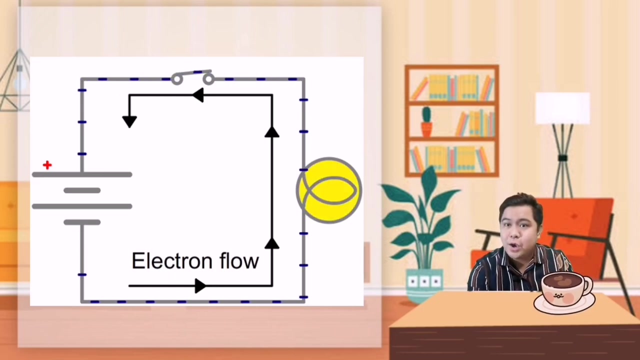 Now, when this happens, a giant spark of lightning is formed. A giant spark of lightning can then start to produce. Now, do you think electricity such as lightning can reach you? Let's study current electricity to answer that. Now, to visualize electricity flow, let's use water coming from the hose as an example. 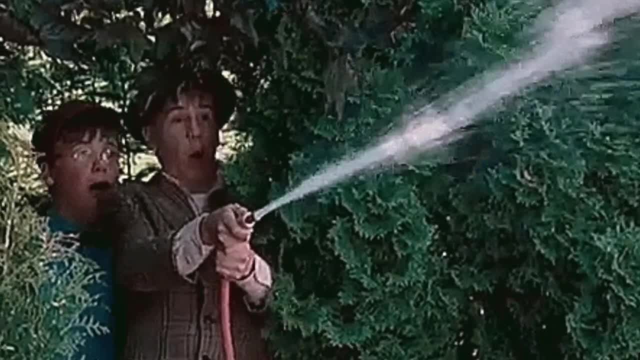 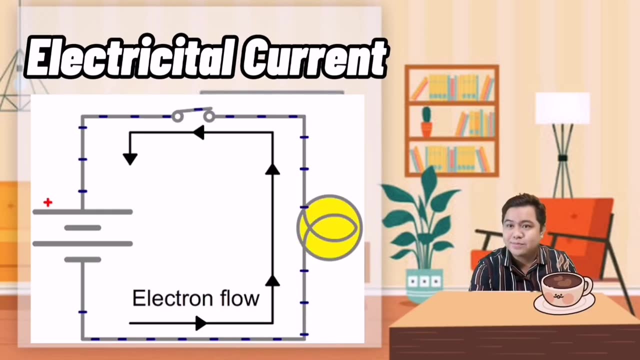 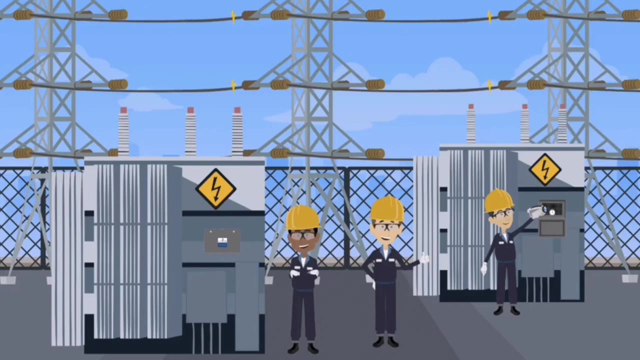 Electricity is like the water flowing through this long tunnel. Now the flowing of electricity flows from the hose. Now the flowing of electricity flows from the hose. electricity is called an electrical current. Currents of electricity flow through power lines, transformers, to the wiring. That's why, from power plants to the wirings, electricity was able to. 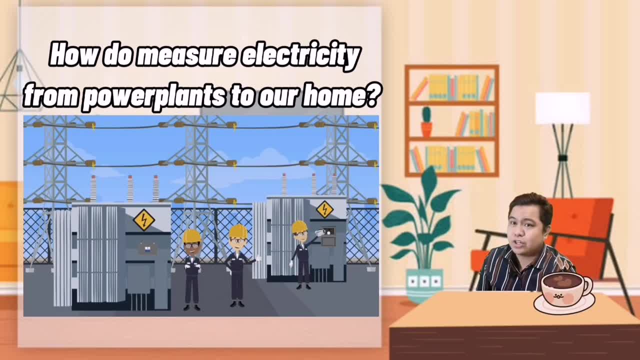 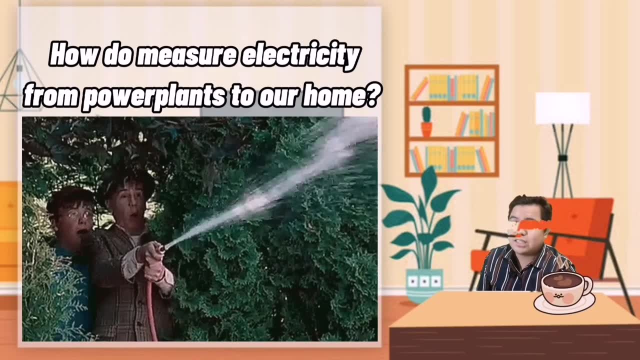 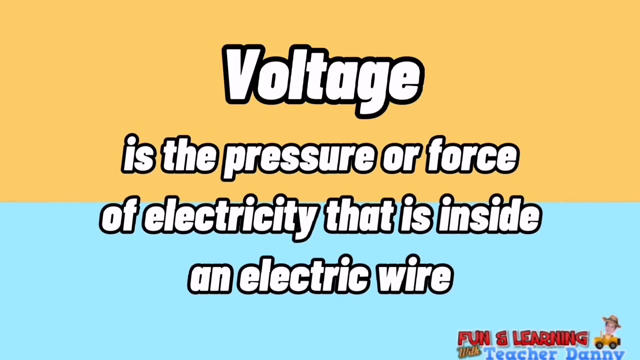 reach our homes. Now how do we measure electricity coming from these power plants to our home? We are going to compare electricity to a garden hose, again with a nozzle. Now, voltage is the pressure or force of the electricity that is inside an electric wire. Now we measure voltage. 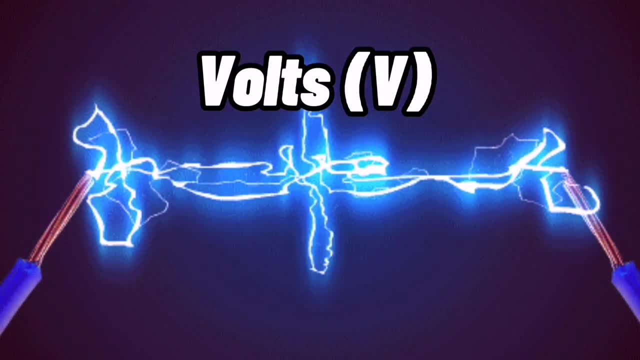 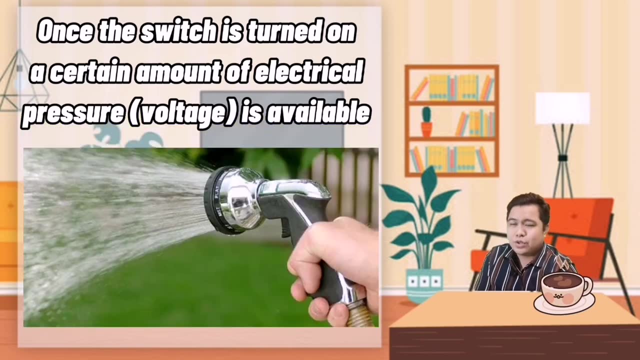 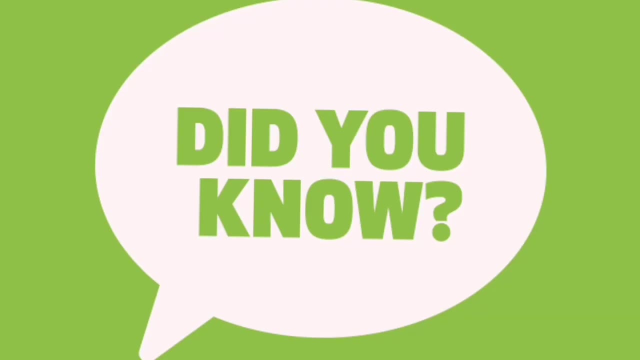 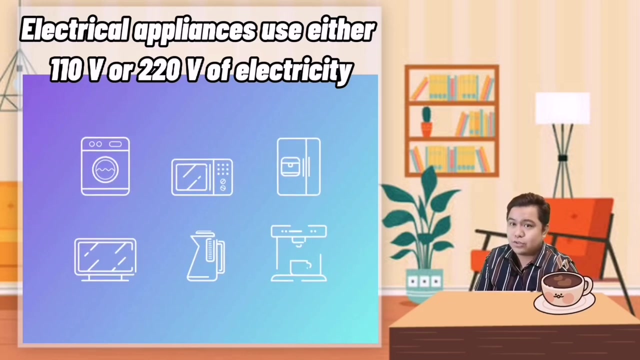 in volts Now, just like the water in a garden hose. now, once the switch is turned on a certain amount of electrical pressure, the voltage is available to be used. Now here's a quick fact: All electric appliances either use 110 volts or 220 volts of electricity. So you better ask your mom and dad first how much. 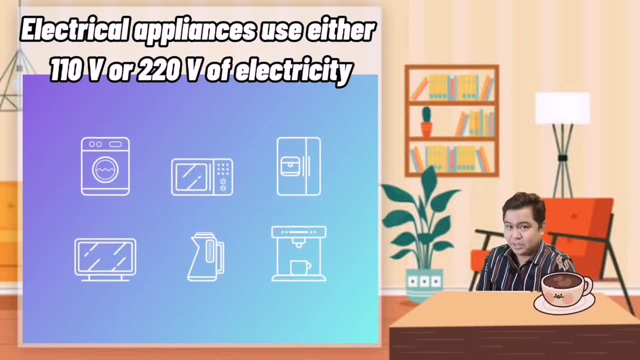 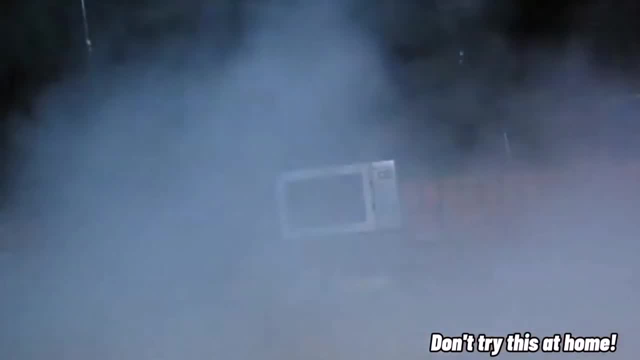 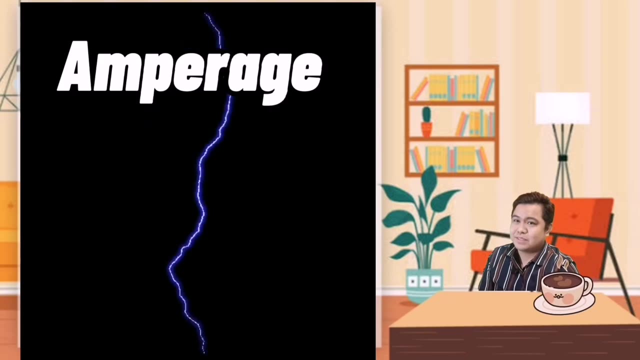 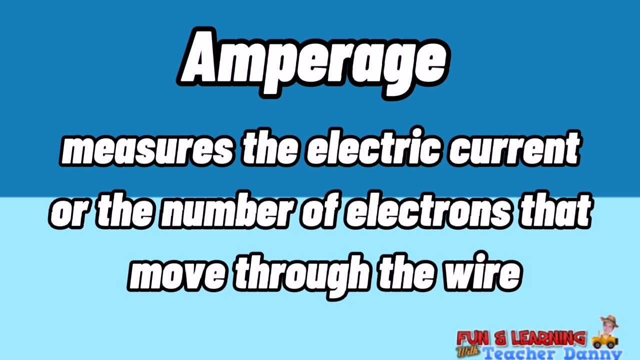 pressure is needed to power up your appliance or else, boom, you might be in danger. Oh no, Now amperage measures the electric current or the number of electrons that move through the wire. Amperage can be compared to the spray of water coming out of the garlic hose. 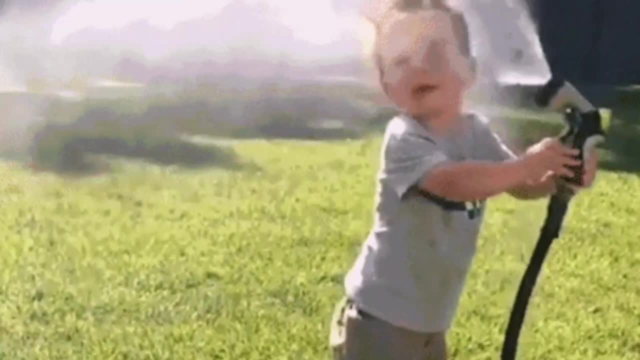 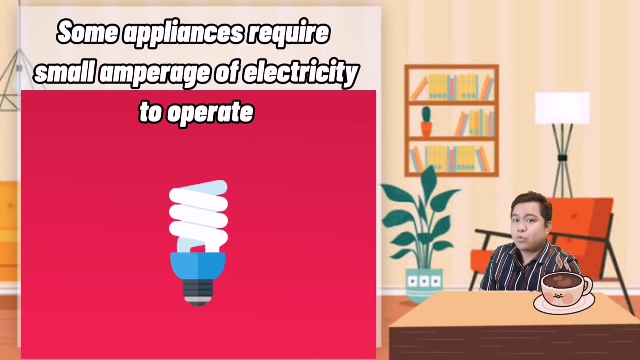 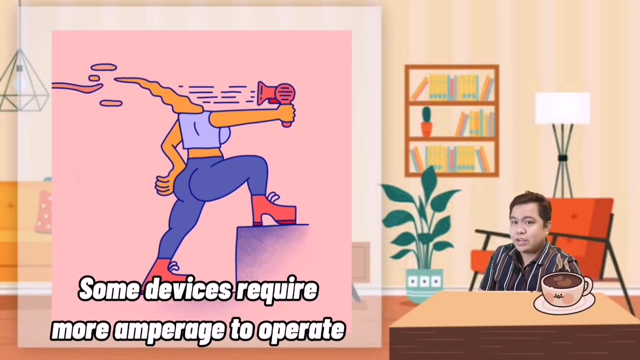 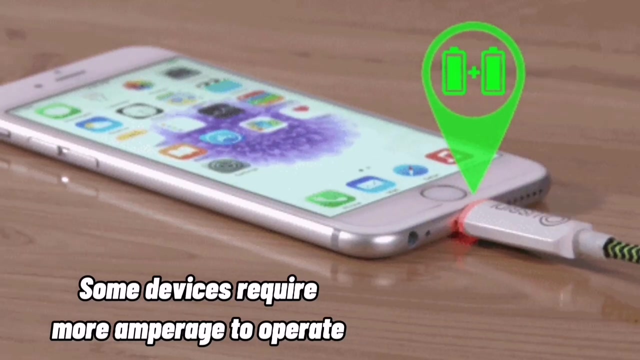 The nozzle can be open just like a little bit, or can be opened a lot. Some electrical appliances, such as light bulb, required a small amperage of will be used to operate, while larger devices like hair dryers, refrigerators and other big appliances require more amperage. now the quantity of electrical energy use is: 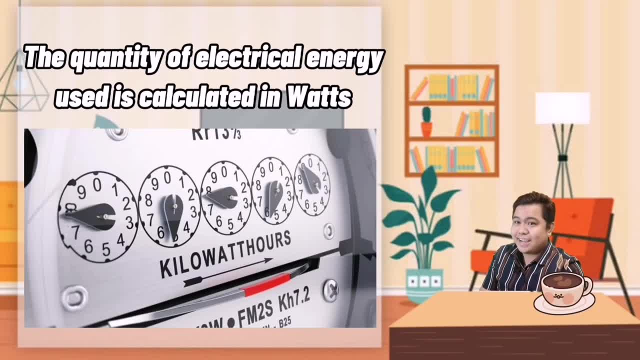 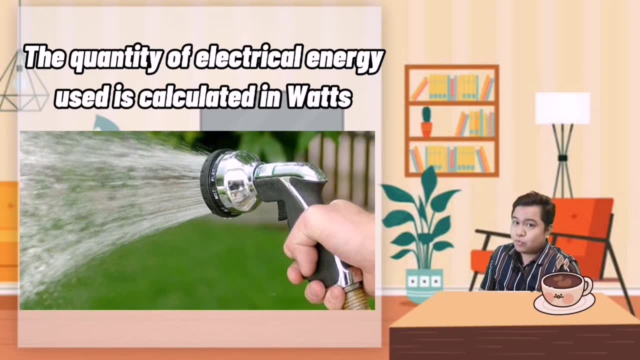 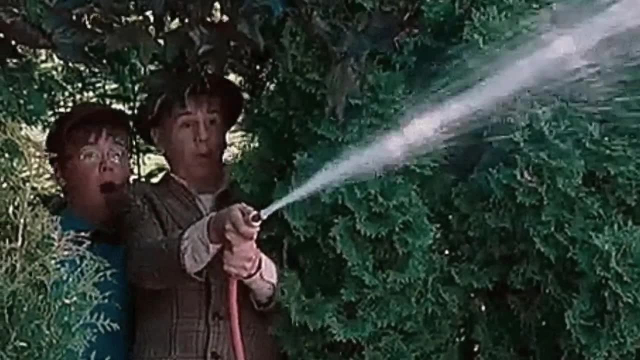 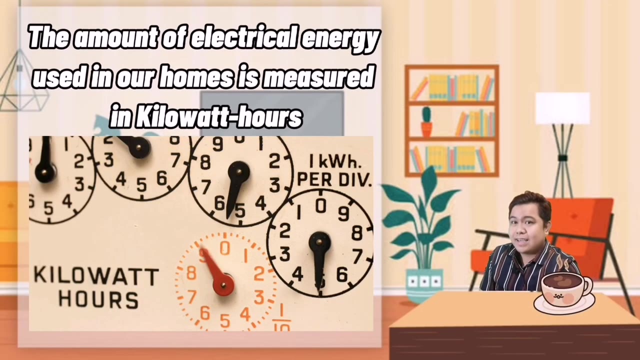 calculated in watts. now. this is like the amount of water that comes out from a garden hose. now, to increase the amount of water flow out of the hose, you can either open top further or increase the size of the opening of your nozzle. now the amount of energy we use in our homes is measured in kilowatt hours. now to 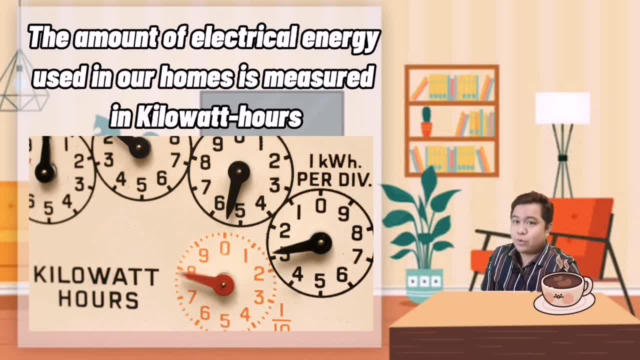 recognize that how much energy is used. when your mom or dad starts to yell at you and say, stop wasting so much energy, it's really that you are consuming a lot of energy. now, speaking of small sources of energy, you can measure the amount of energy that you use in your house and 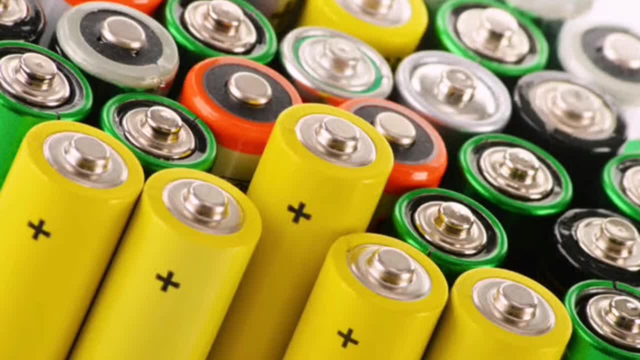 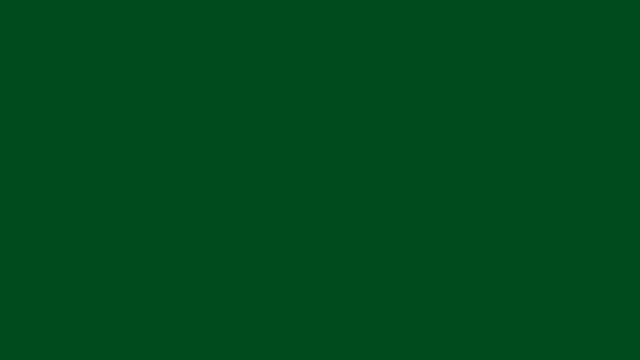 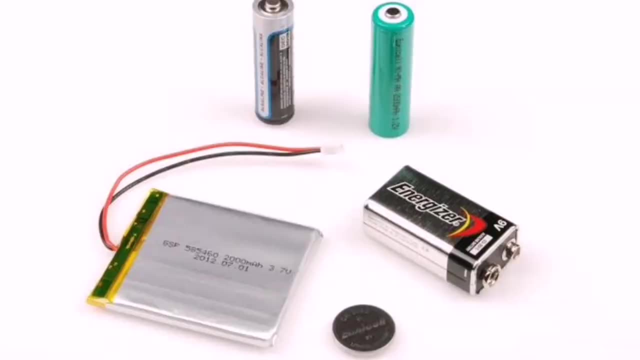 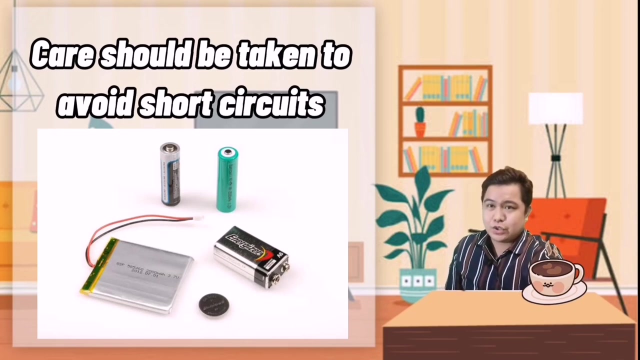 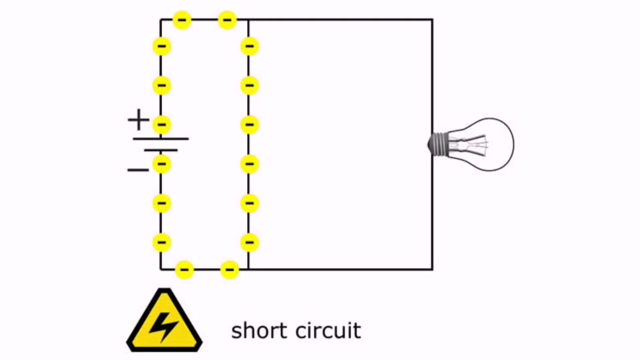 electricity. a dry cell can store electricity, such as this small batteries. these are relatively safe sources of electricity. now these are used for experimentation and study, but care should be taken to avoid short circuits. now this short circuits are when wires heat up and waste energy. this can occur if too much amperage are getting pulled through household wires. now. 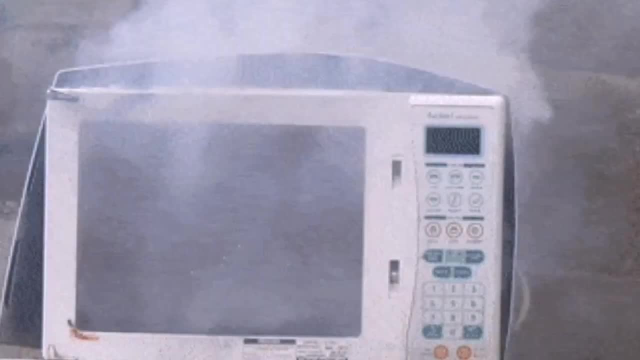 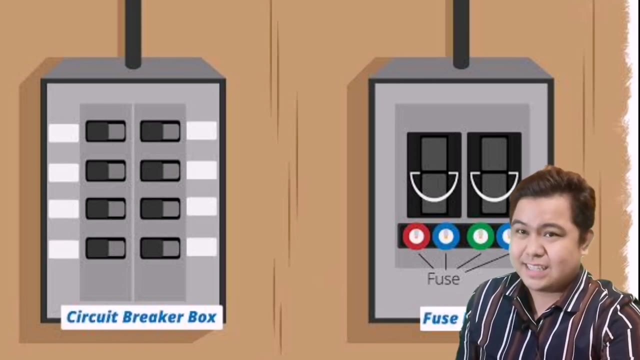 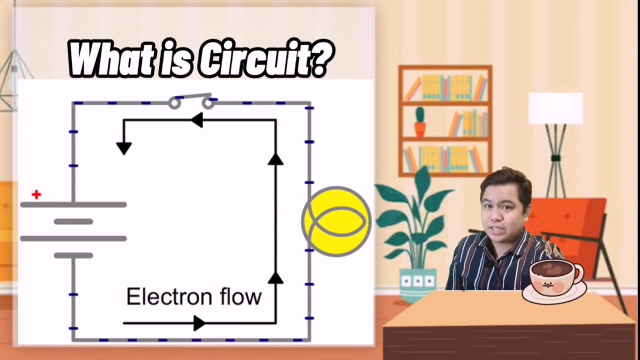 this can cause fire. houses have circuit breakers and fuses to control busting of appliances. now wait, what is circuit? by the way? now try to open your light. what part of the circuit would you go first to open it? yes, the most familiar part of the circuit we know. 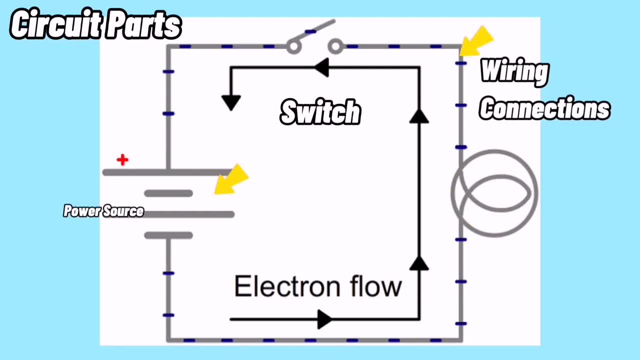 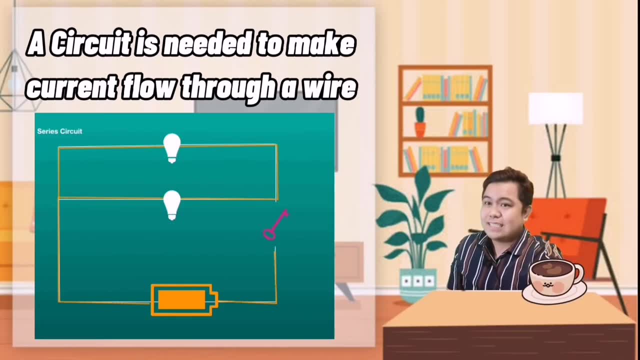 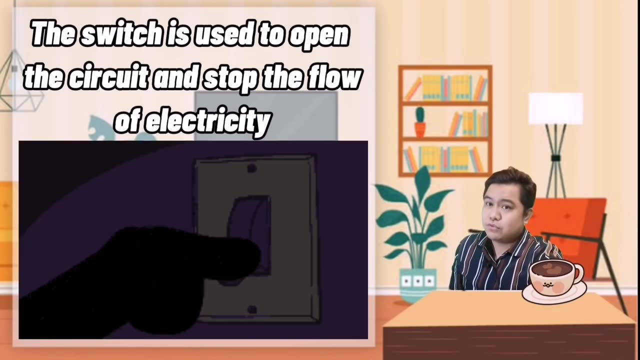 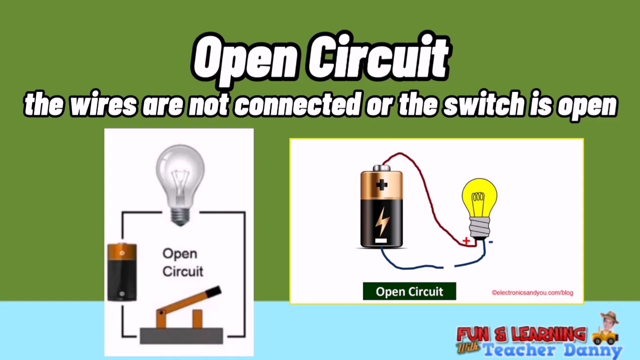 switch. but without wiring connections our source and loads, we cannot make electricity flow. now a circuit is needed to make current flow through a wire. the switch is used to open the circuit and stop the flow of electricity. in an open circuit, wires are not connected or the switch. 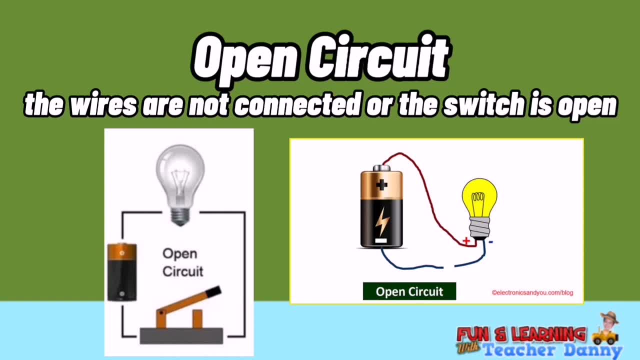 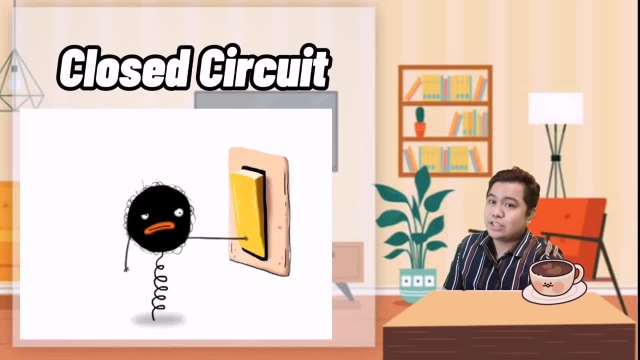 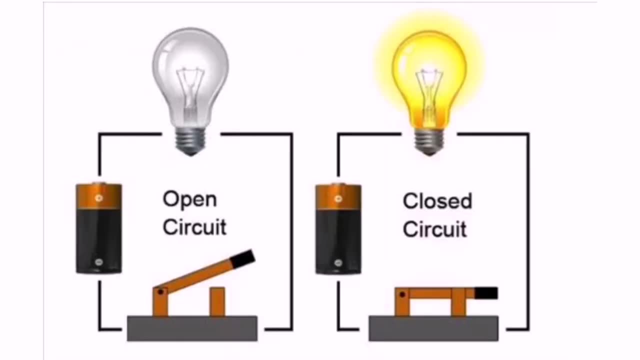 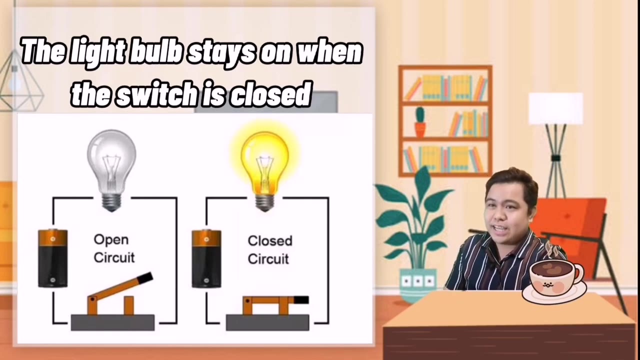 is open, this means that electricity will not be able to flow. closing the switch allows electricity to continue its flow. this is a closed circuit. the light bulb stays on while the switch is closed. wait, hold on there. this is quite confusing because we are used of saying open the switch to turn on. 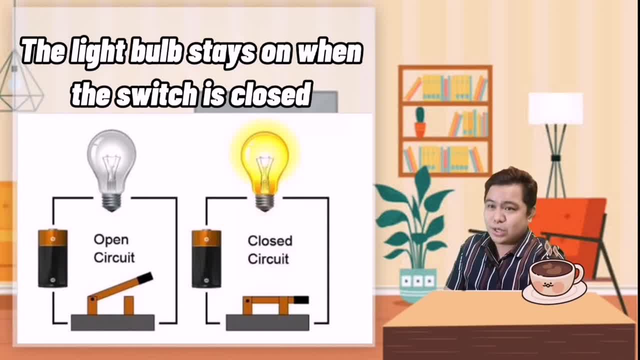 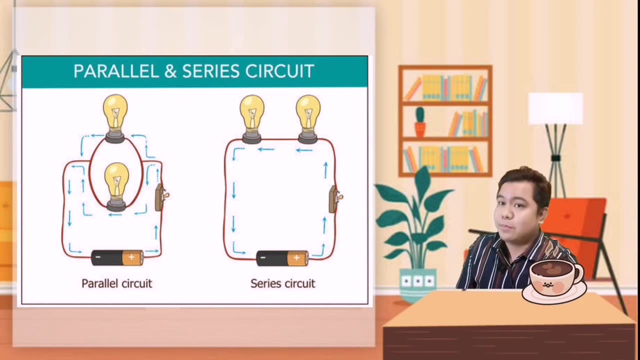 the switch of a circuit. if the switch is closed or it is aligned in the wiring, the load or the light bulb will operate. now there are two types of circuit: the parallel and the series. now, what's the difference between the two types? now, first, in a parallel circuit, each of the bulbs, or we call, 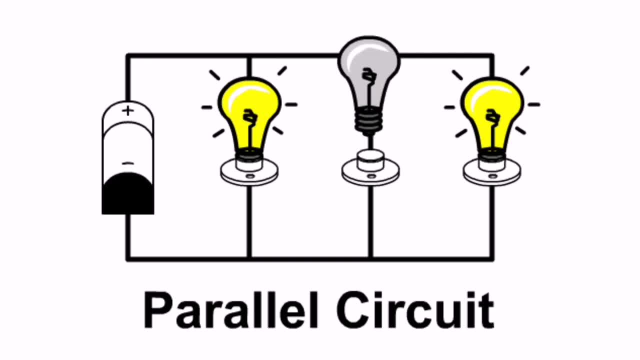 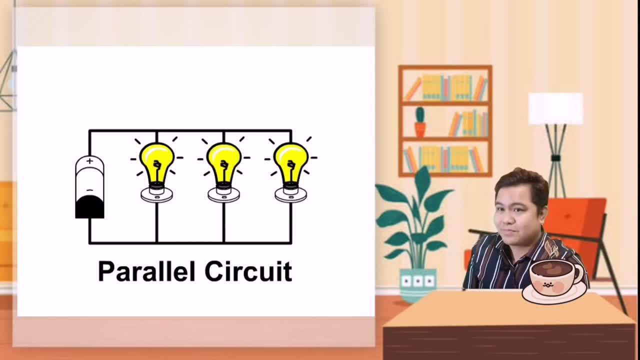 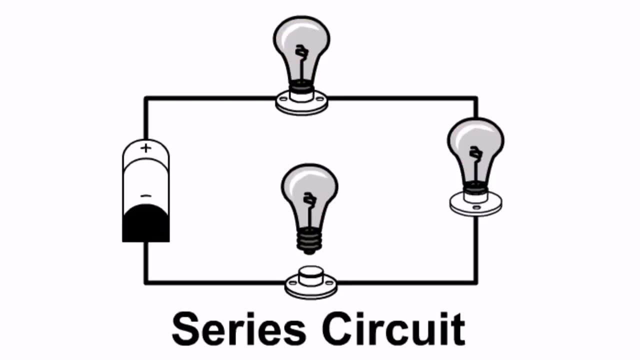 is directly connected to the power source, which means if a bulb is removed or burnt out, the other bulb will still work. but in a series circuit each of the walls or loads is connected in a circle or one path. now this means if a bulb is removed or burnt out, the connection is damaged and none of the lights will die. 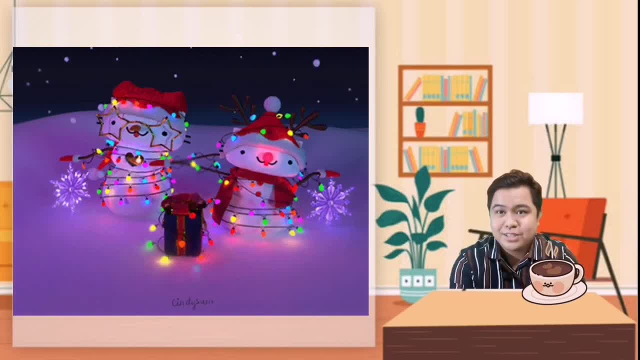 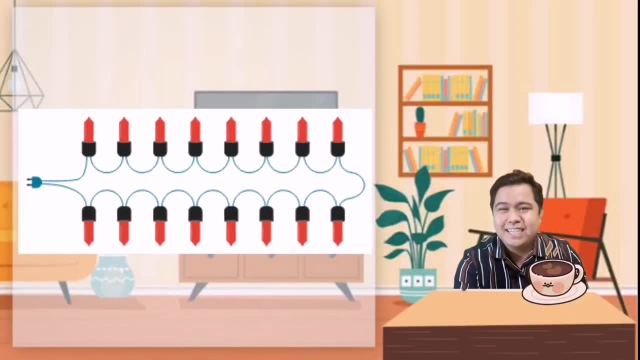 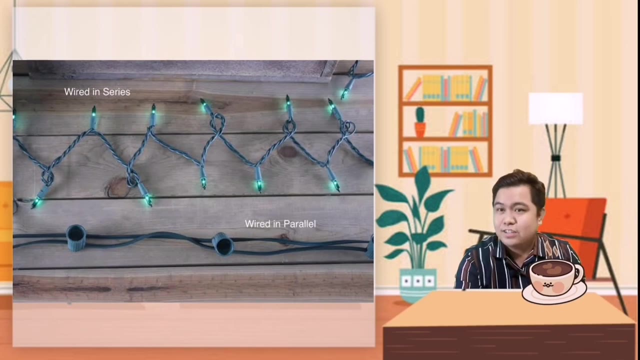 now. a example of this is our christmas lights. some of our christmas lights won't operate if one bulb is missing or damaged. this is a serious type of christmas light, so if you don't want to hustle on this, try purchasing parallel now. can you differentiate now the two types of circuits? 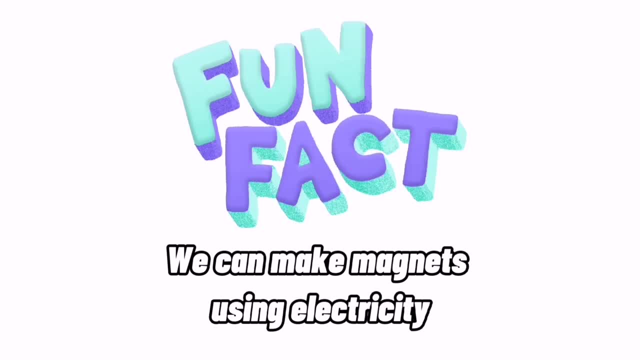 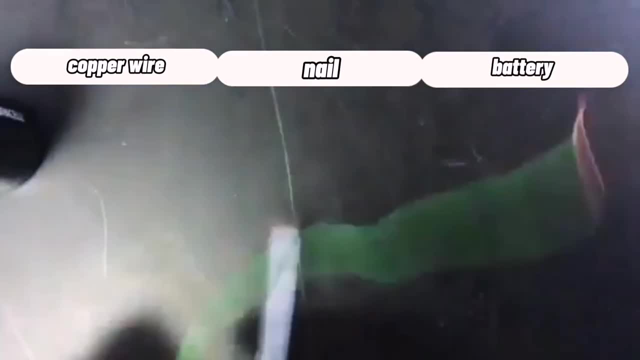 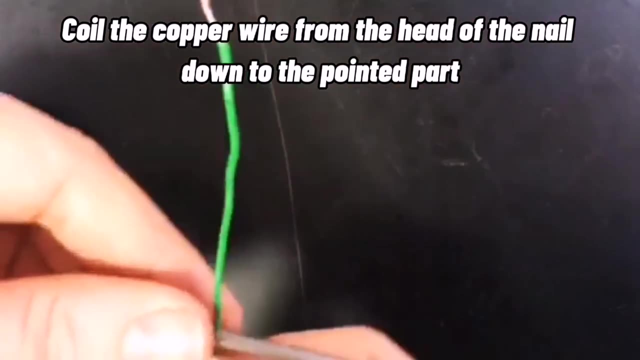 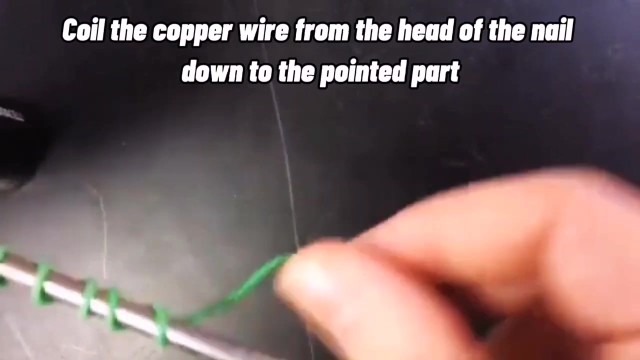 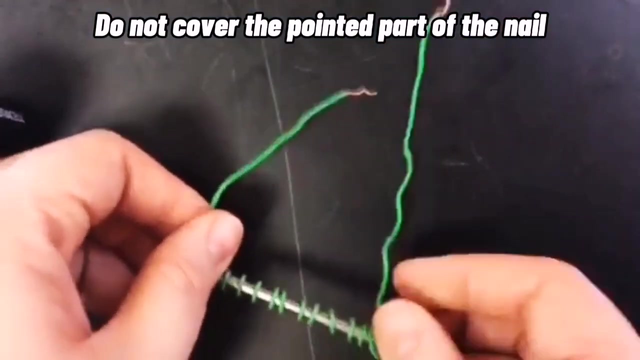 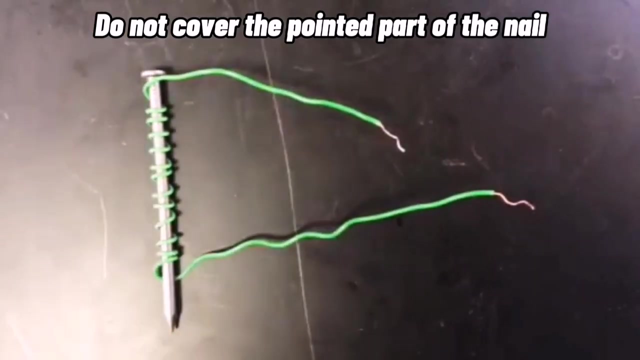 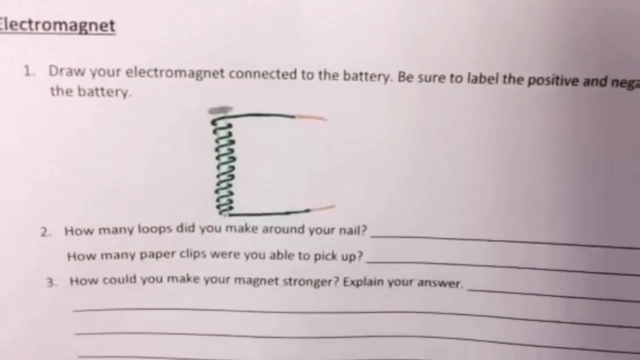 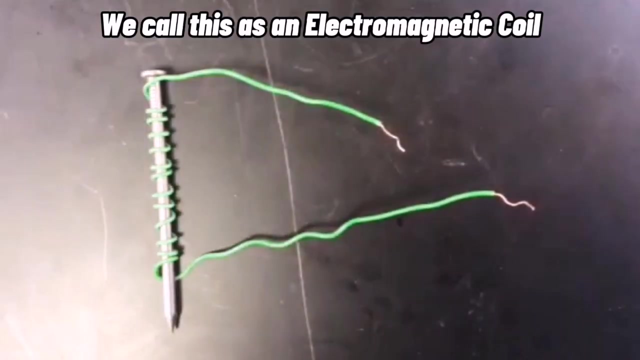 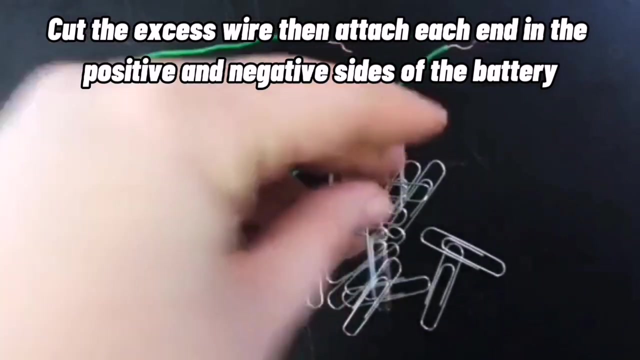 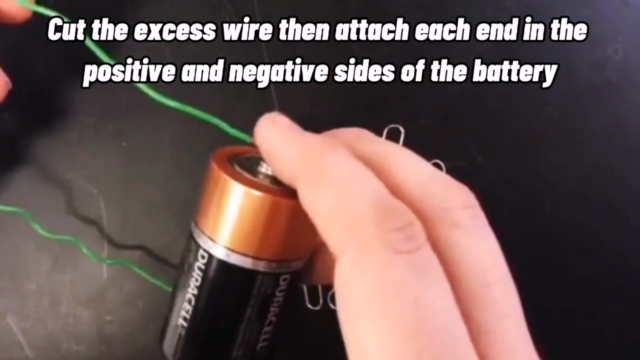 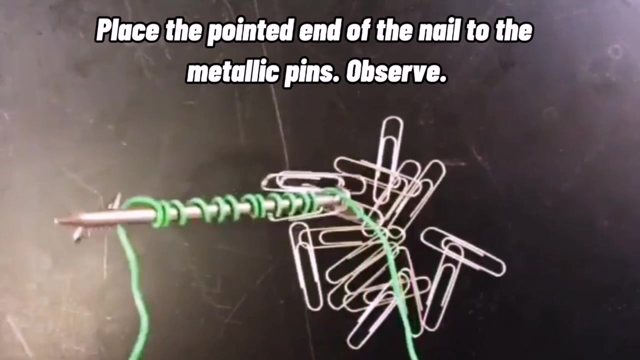 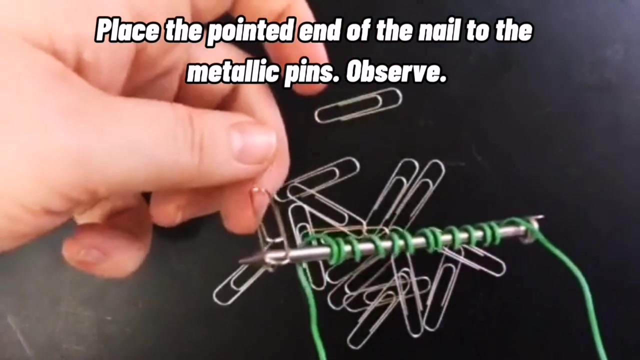 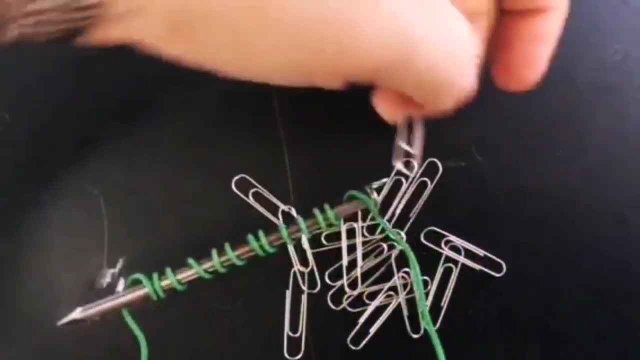 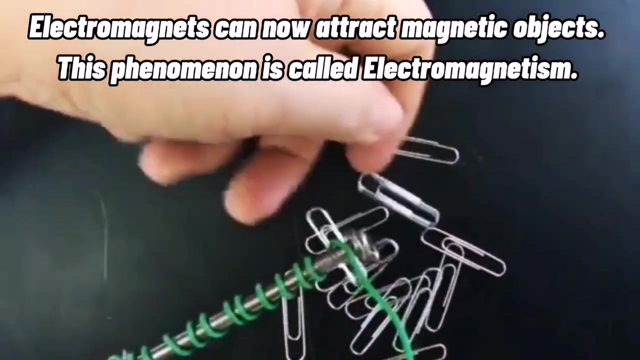 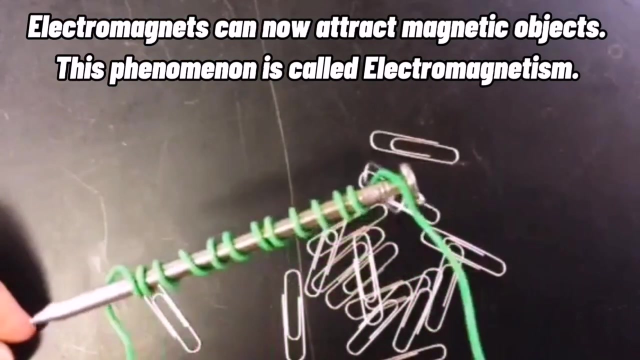 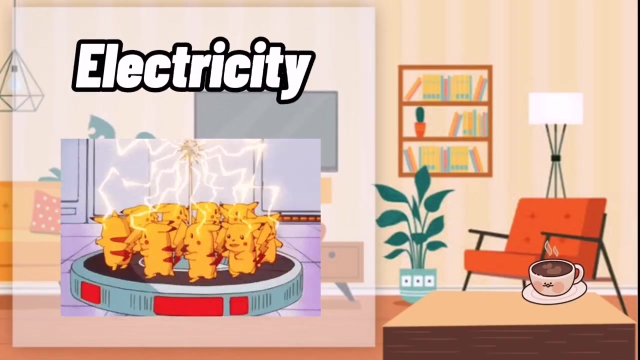 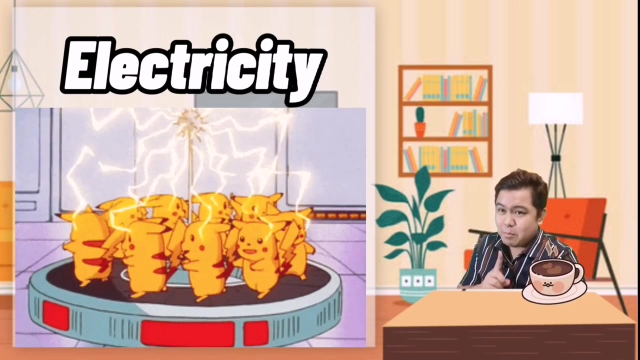 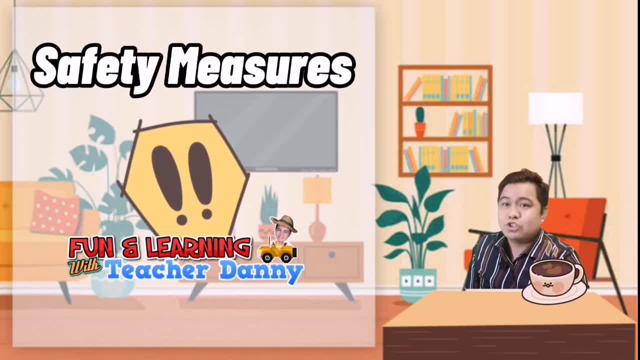 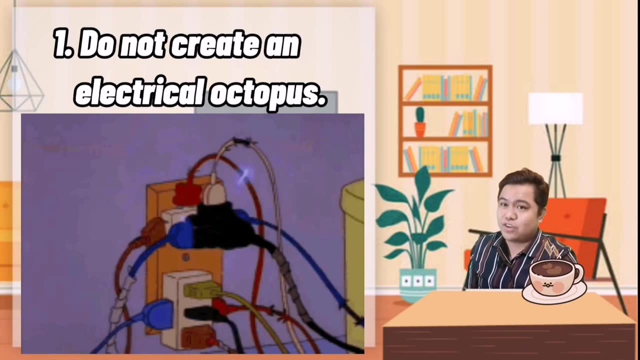 Now here are some safety measures from Teacher Danny to prevent yourself from being electrocuted or having trouble with electricity. First, do not create an electrical octopus. Only use the standard number of plug-ins provided. Number two: always unplug electrical devices before cleaning or repairing. 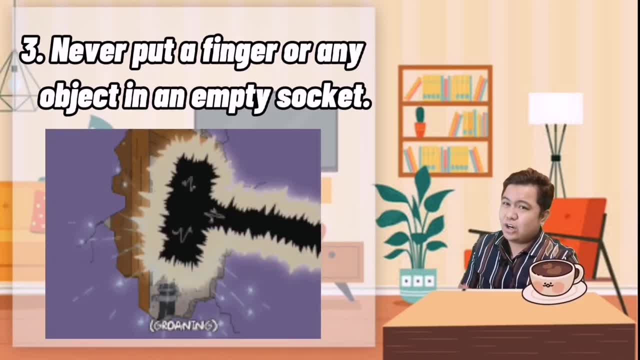 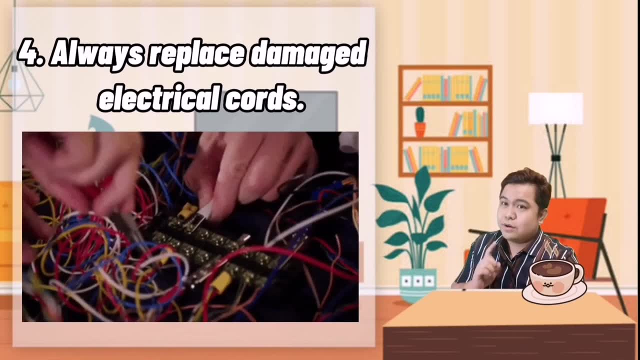 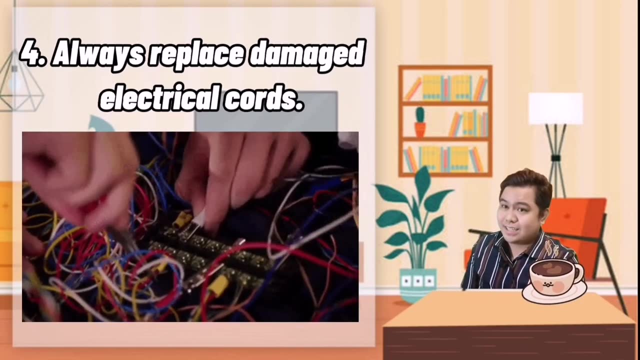 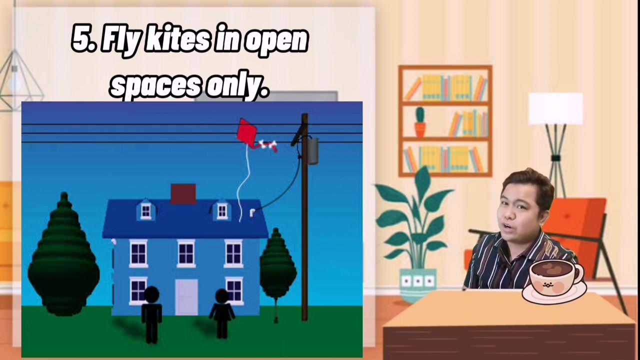 Three: never put a finger or any other, Most especially those conductors in an empty socket. Four: always replace damaged cords, But since you are young, ask your parents for help regarding this. Five: fly kites in open spaces only and watch out for electrical wirings outside. 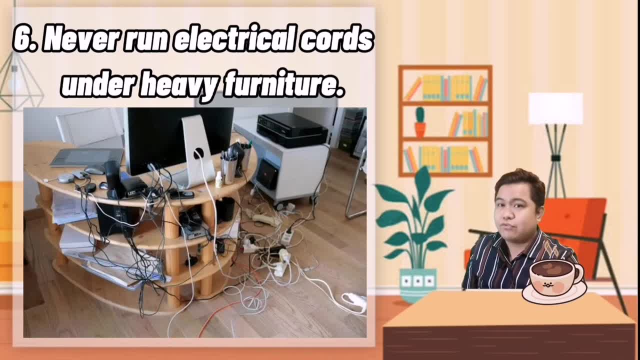 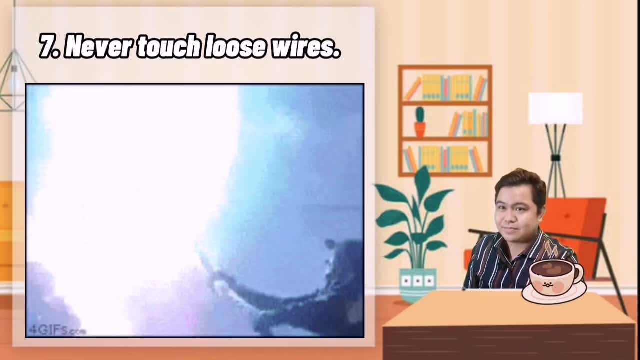 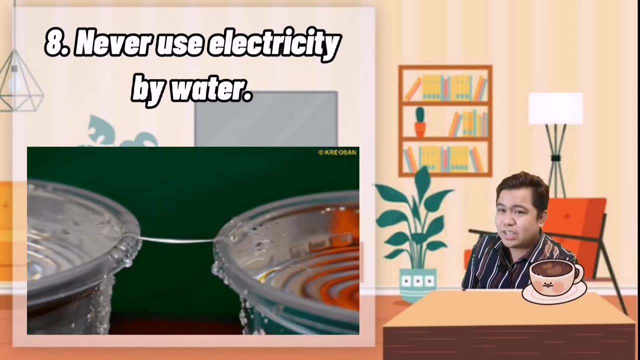 Six: never run cords under heavy furniture. Seven: never touch loose wires. Eight: never use electricity by water. Remember our lesson on conductors and insulators. If you have missed that, better watch it again. I'll place the link here. 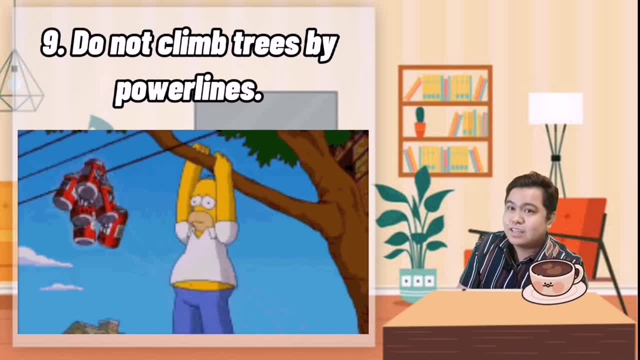 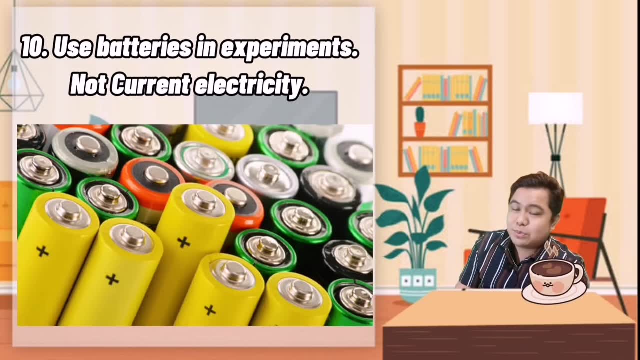 And nine: do not climb trees by power lines. That is not safe and you are not a monkey. And ten: when you do experiments, only use a power line. When you do experiments, only use batteries, never in the current electricity. 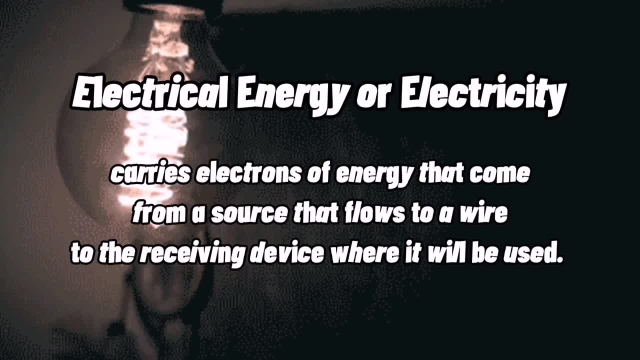 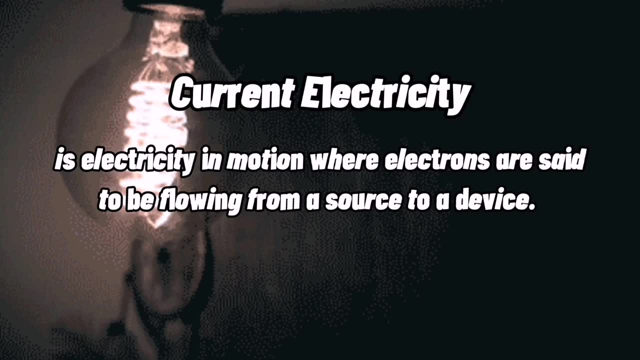 So remember, electrical energy, or electricity carries electrons of energy that come out from a source that flows to a wire, to the receiving device where it will be used. Current electricity is electricity in motion, where electrons are said to be flowing from a source to a device. 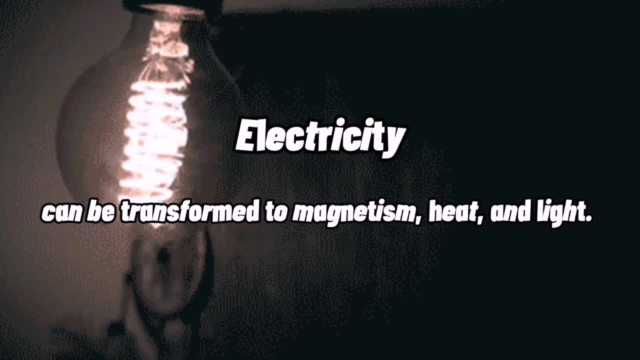 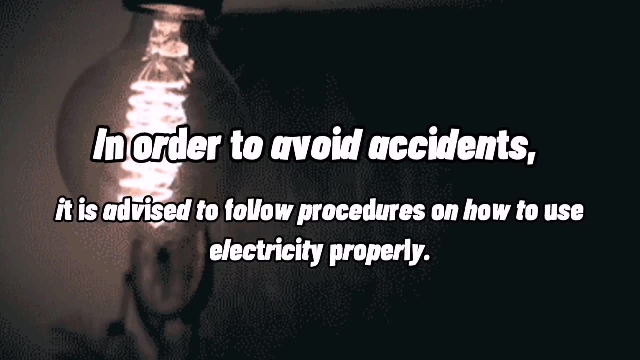 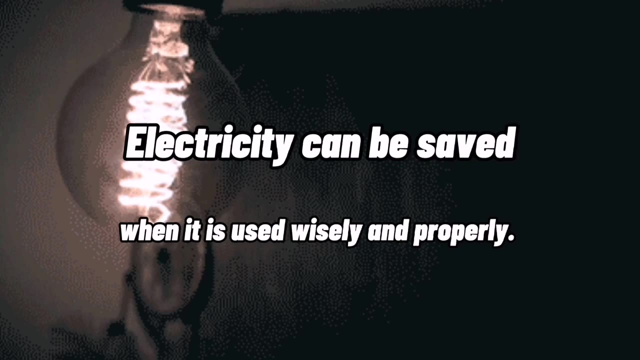 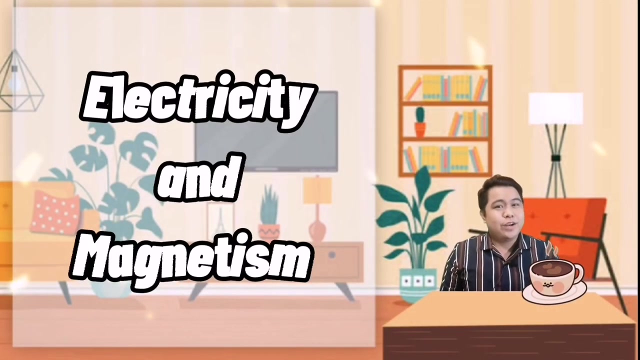 Electricity can also be transformed to magnetism, heat and light, And, in order to avoid accidents, it is advised to follow procedures on how to use electricity properly. Electricity can be saved when it is used wisely and properly. Thank you very much for joining our wonderful adventure in the world of physics.